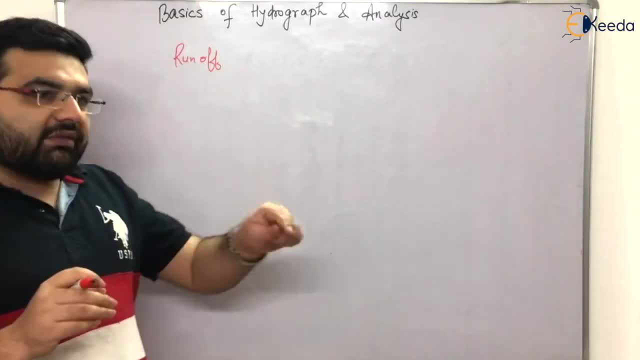 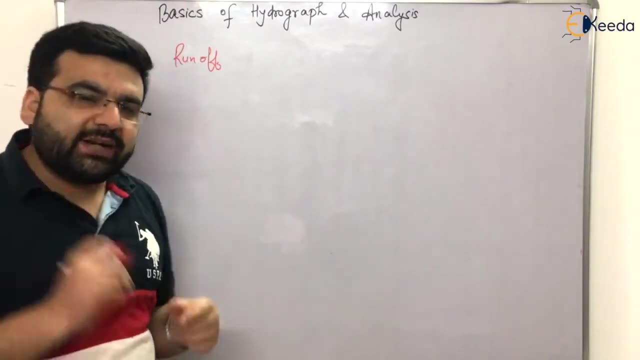 initial losses, the depression losses and everything right. Whatever the volume of water you are left with or whatever the depth of precipitation you are left with, it results into Runoff. Simple, right. So Runoff is of two types. One: we have a long-term Runoff. 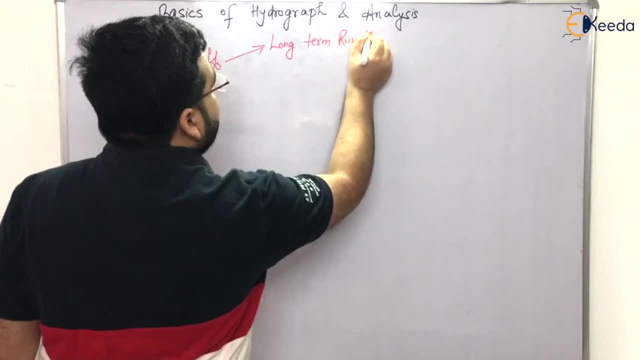 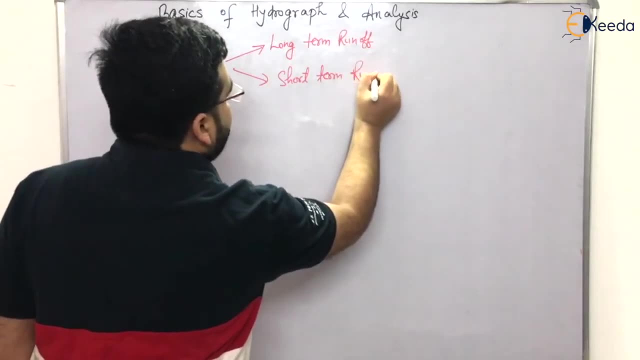 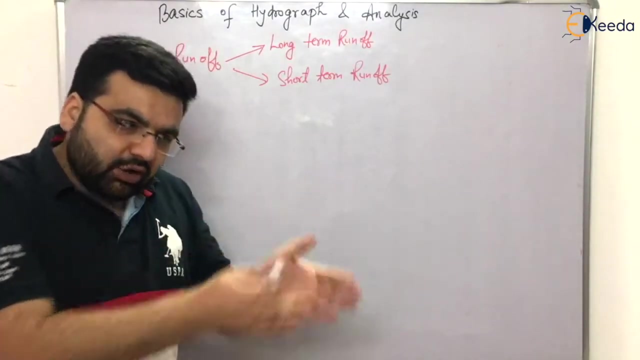 Long-term Runoff And one we have short-term Runoff, Short-term Runoff. Now, what is this long-term Runoff? So, long-term Runoff means the Runoff which is actually happening over a long period of time. Let us say it is the Runoff in a river right Or the Runoff in a canal right Which 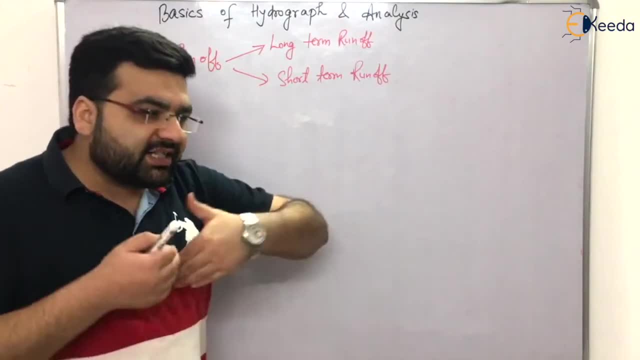 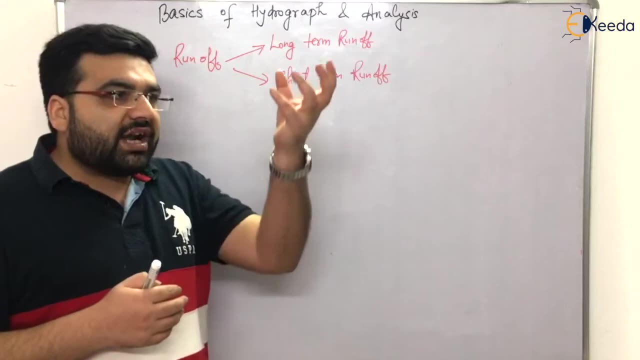 is happening over a period, over a course of time. right, That is a long Runoff, right Now. long-term Runoff. let us say short-term Runoff, right In Long-term Runoff. suppose that a storm has happened, right? Or you can say a storm has just arrived over a particular catchment area. 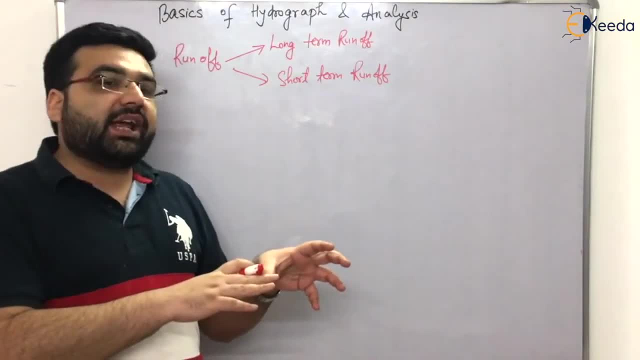 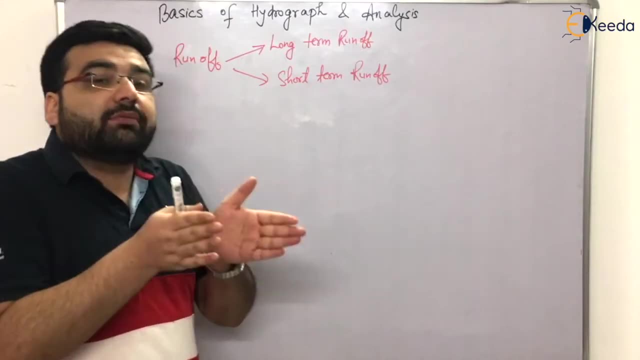 So when the storm, the storm will be giving all its precipitation, then at a particular gauge station, you will be observing a certain peak that will be only for a short term, only for a short period of time. So that type of Runoff is known as. 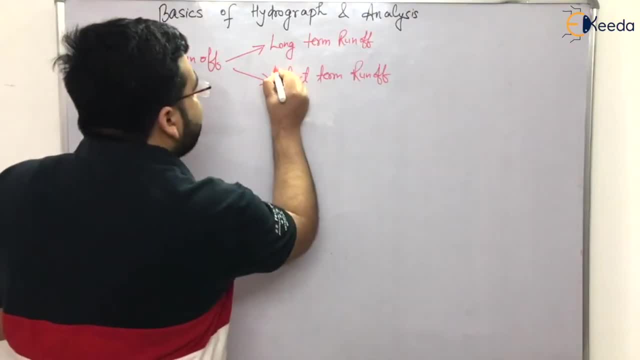 short-term Runoff. So in Hydrograph analysis, We are basically discussing the short-term Runoff, only right. Long-term Runoff: we are not discussing the short-term Runoff, but we will keep하기 the short-term Runoff only right. 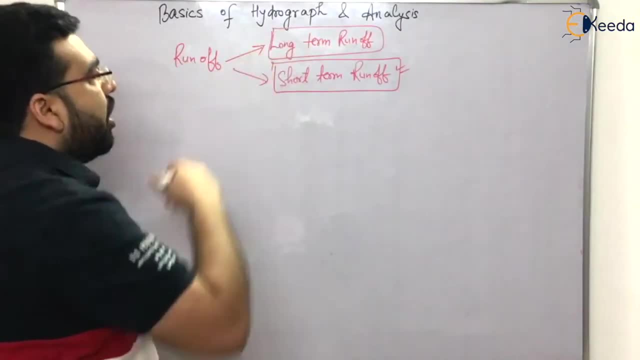 In Long-term Runoff we are not discussing the short-term Runoff. so in Hydrograph analysis we are basically discussing the short-term Runoff. only right, we are not discussing in hydrograph, but for long term runoff we are discussing the stream. 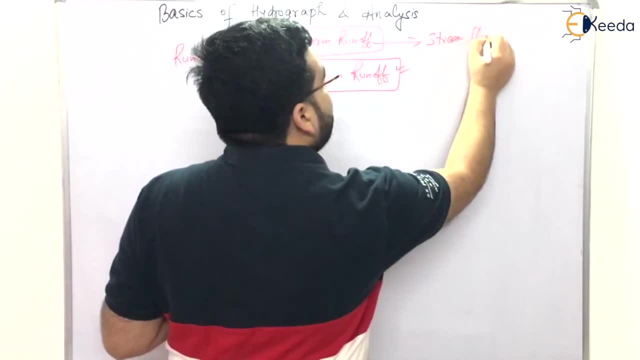 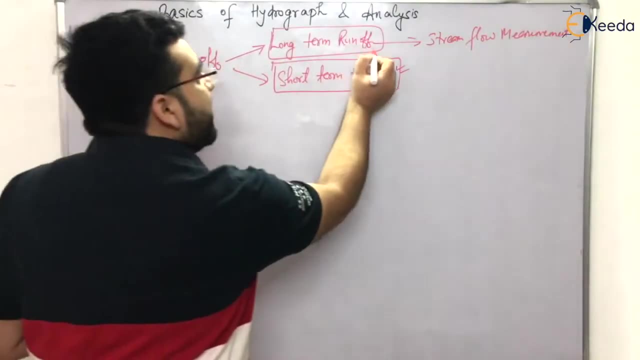 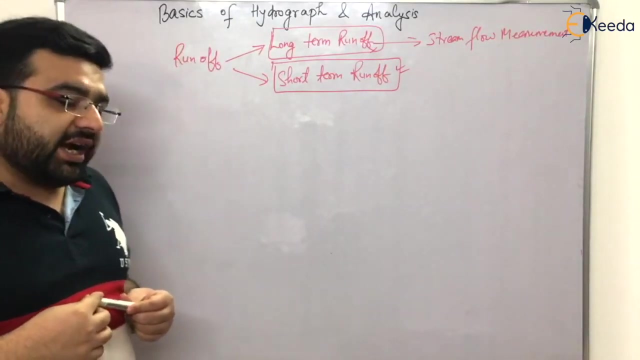 flow measurement, stream flow measurement or stream flow hydrology- right, but that is not in our syllabus. earlier it was in GATE syllabus. if you look at the past 25 years of GATE examinations and the syllabus of GATE examination up to 2010 or 11, so this was in syllabus, right. 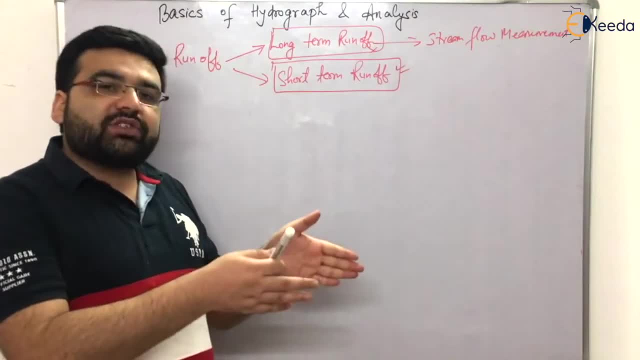 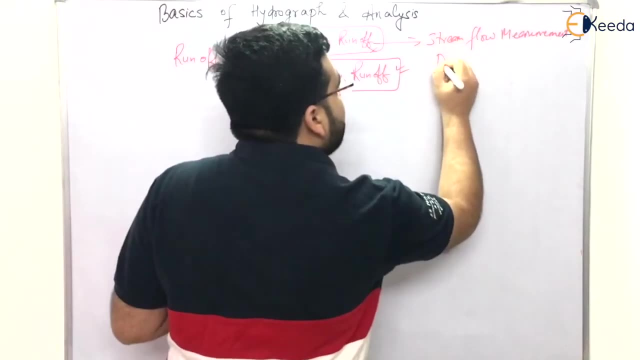 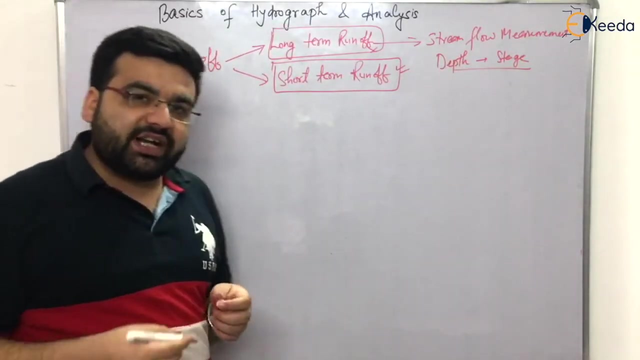 so you must be observing some numericals based on the velocity of stream flow and the discharge of stream flow. right, the depth, the stage, also known as depth. right, so depth is also known as stage, depth is also known as stage. right. so stage, discharge relationship and other topics right, but nowadays the GATE has, you can say, eliminated this topic from. 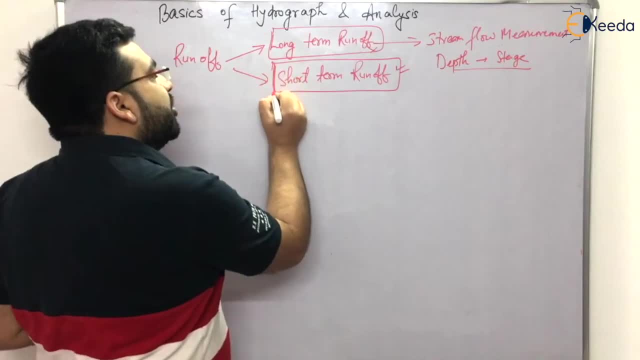 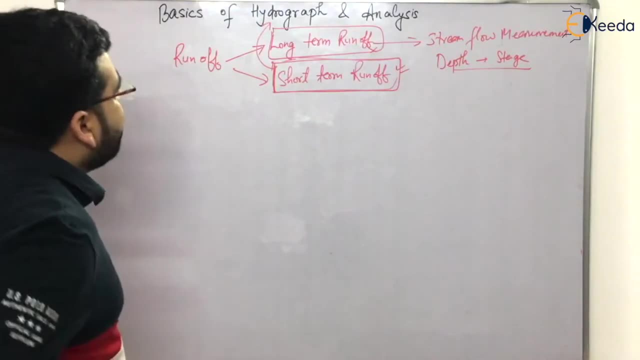 the syllabus of GATE examination. so we are only left with the short term runoff in which we will be studying the hydrographs right Now. first of all, let me tell you what a hydrograph is. now, to make you understand what a hydrograph is, first of all, let me draw over catchment area. right, let us say this is a catchment. 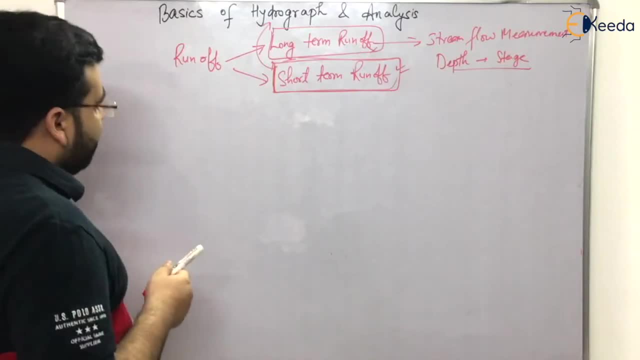 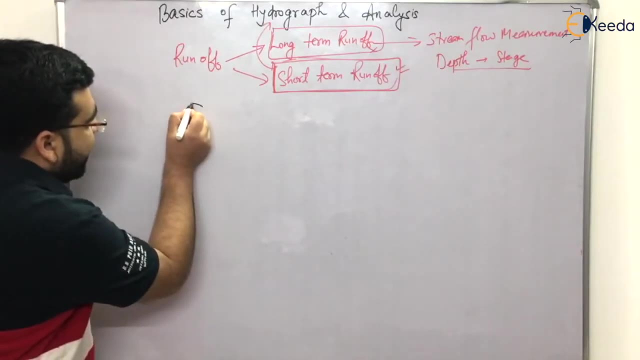 area. let me take the black marker to make you understand more precisely about the catchment area. so let me take one catchment area. let us say this is a catchment area, this is a catchment area, this catchment area, we have a streams right. let us say that is a main. 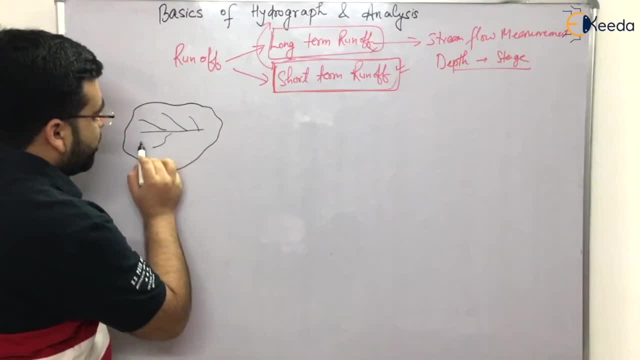 stream. these are the tribute reels. right, this is the normal stream. serious stream. reduce stream balance. this treatment points, and here we are able to draw mirror of field toít particular area. these we have, sample distribution of the fluid type, of the liquid partisan flow. these are the tributaries, let us say right, and this is a particular catchment. 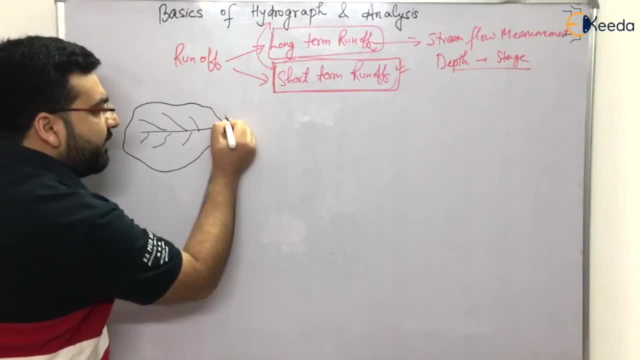 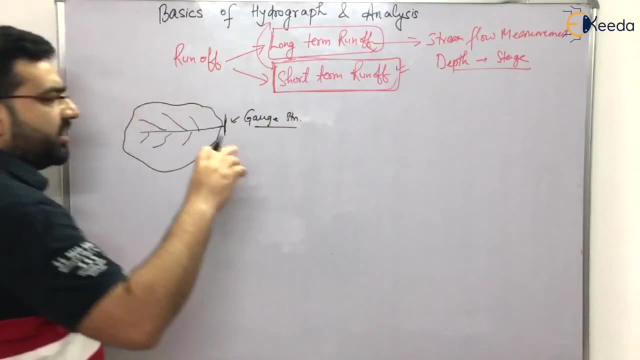 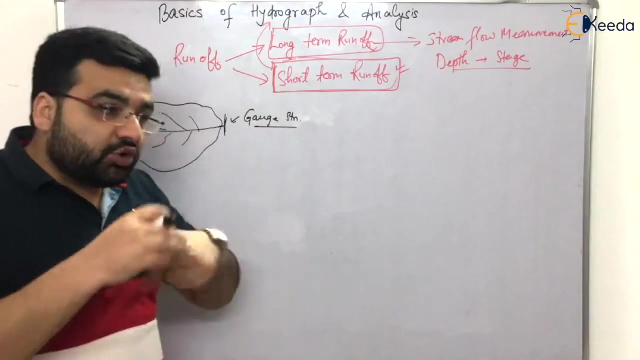 area and the exit of this catchment area, we have placed a gauge station, gauge station, gauge station, which will measure the stage, or known as a depth also, which will measure depth, which will measure the, you can say, the peak of the discharge, the total discharge, the velocity of discharge. so we have 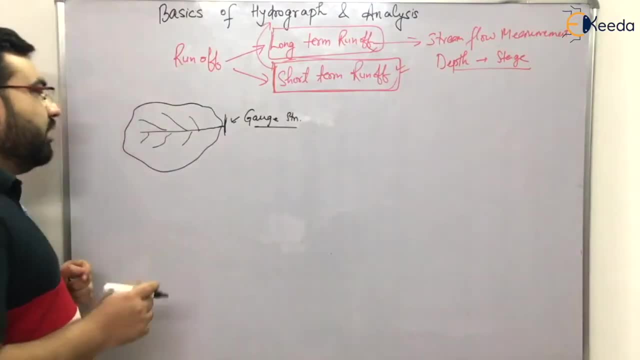 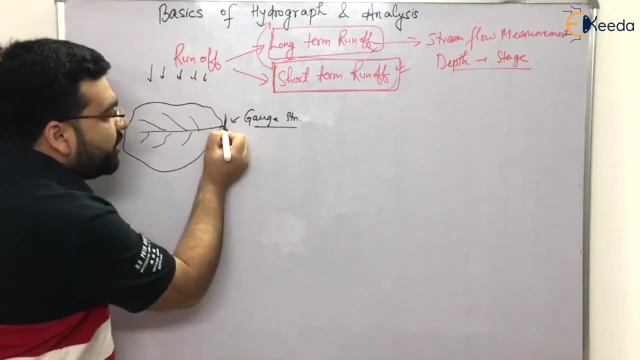 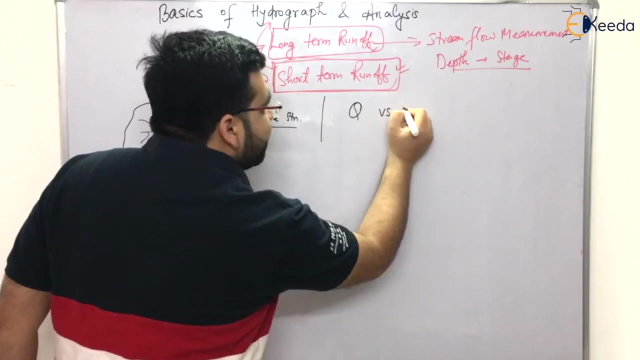 established a gauge station there. simple, yeah, now when precipitation is happening over this area? when precipitation is happening over this area, now what will happen to this gauge station? so if you draw a graph between discharge versus time, discharge versus time, and you are sitting at the gauge station and you are 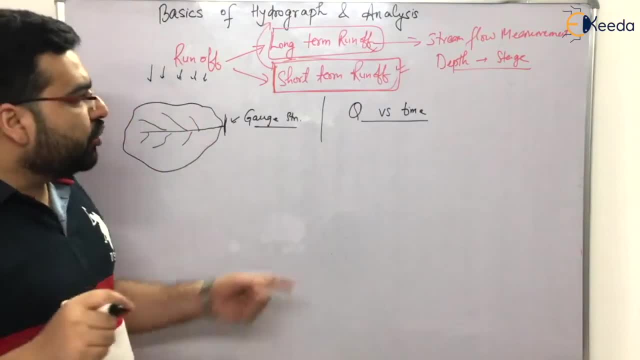 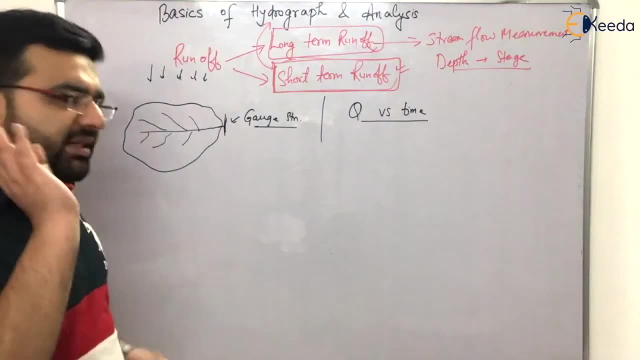 drawing a graph between your discharge and your time to measure discharge. there are a lot of, you can say, methods, some rational methods, some irrational methods. slope area method is also there. lot of methods are there, right- I'm not going, indeed, in that- direct and indirect methods, right. so to measure discharge, a lot of. 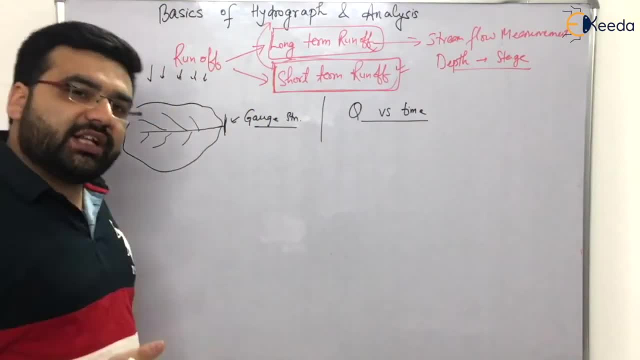 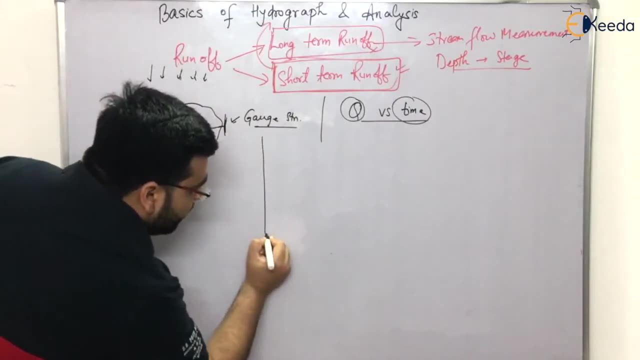 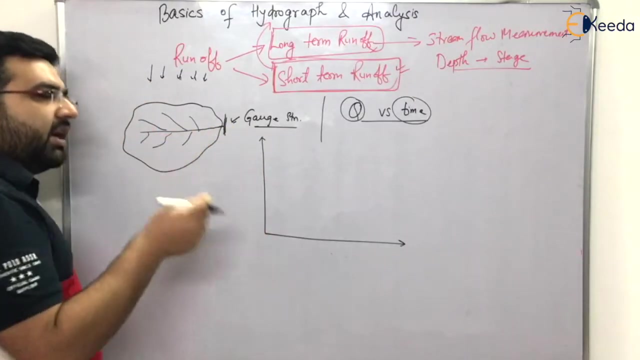 methods are there. now you are sitting at the gauge station, measuring the discharge and drawing a graph between discharge versus time. your graph would be like this. your graph would be like this: now, initially, the this, for example, this stream, it already has some flow, let us say, even without the storm, even without 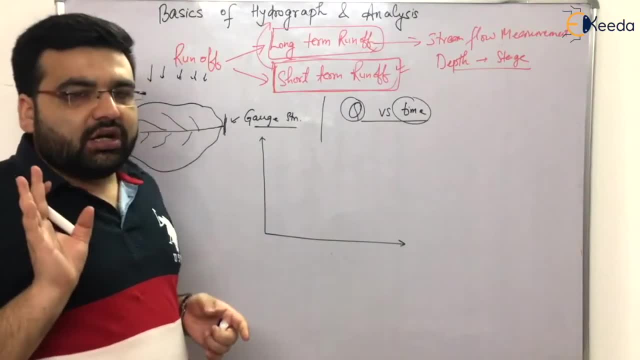 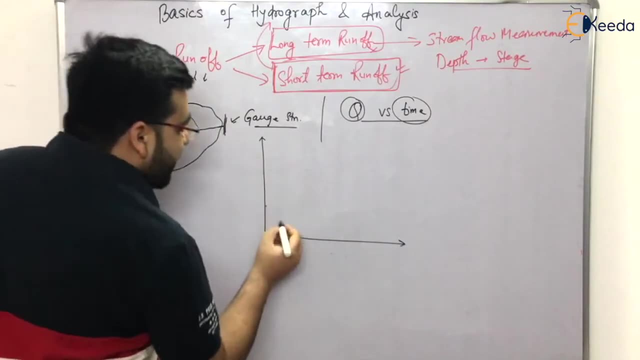 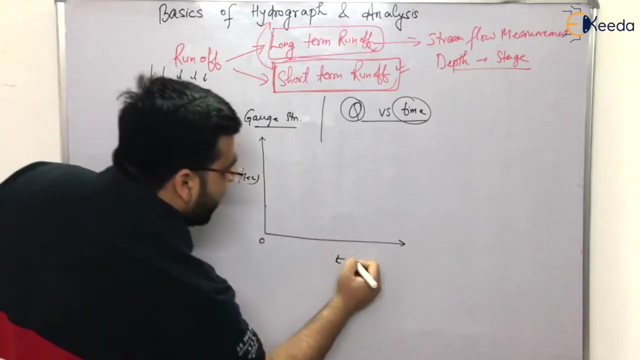 the falling of the storm precipitation, there was, let us say, some discharge in the stream here, right? so some discharge was there, was there right now when this storm has happened. let us say that this is time 0. this is a time depends on the discharge in meters cube per second. meter cubes per second and your. 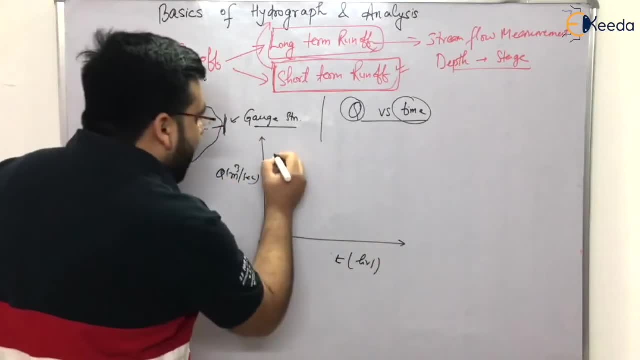 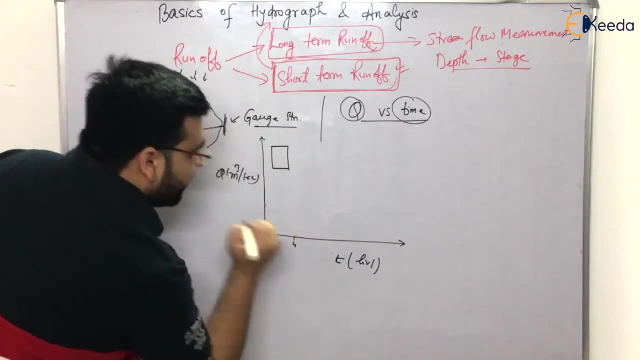 time is in hours. it is in hours right now. this particular storm has happened. let us say between time: t is equal to this, 2 to T is equal to 4. it is just a 2 hour storm. right, DR storm, DR storm. but for time being it is 2 hour storm. great, that's it. 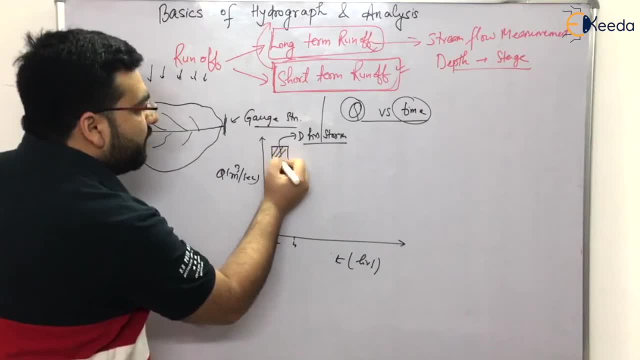 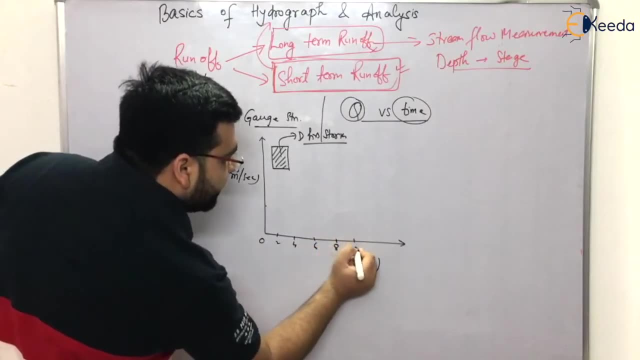 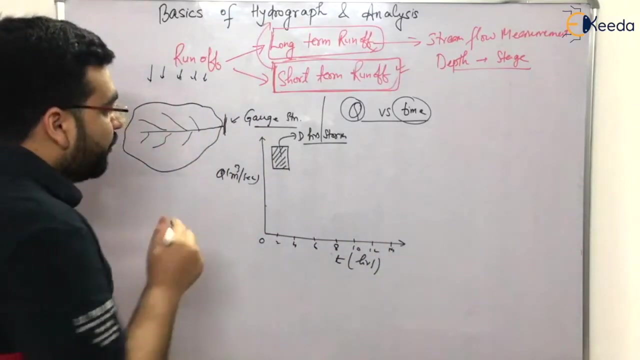 just a 2 hours storm. for 2 hours, this storm has happened over this particular catchment area. what is the area of catchment that I don't know. right, 4, now, 6,, 8,, 10 hours, 12 hours, 14 hours and so on. but this storm has lasted only for 2 hours, right? so what will? 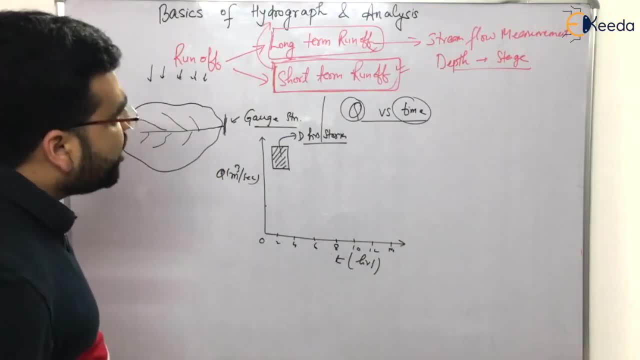 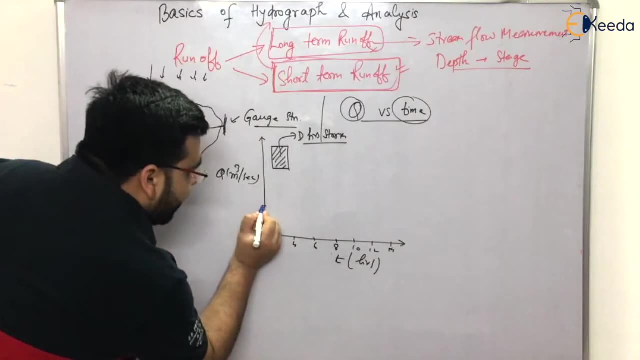 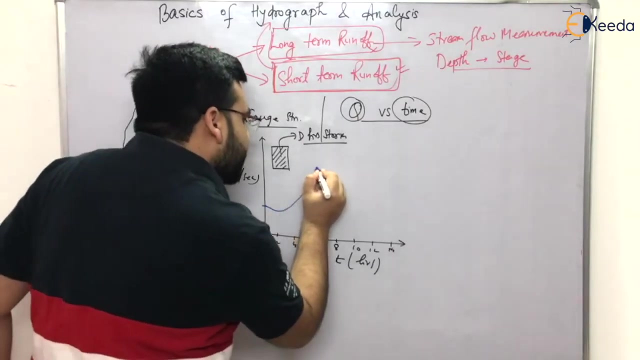 happen at this gotch station. so if you draw a graph between discharge versus time, this is my common sense- that gradually, the discharge will increase. right, so, gradually now. this was the base flow. now, what is this I am explaining now? gradually, sorry, the discharge will increase. it will attain a peak. I don't know at what time it will attain a peak, and after sometime. 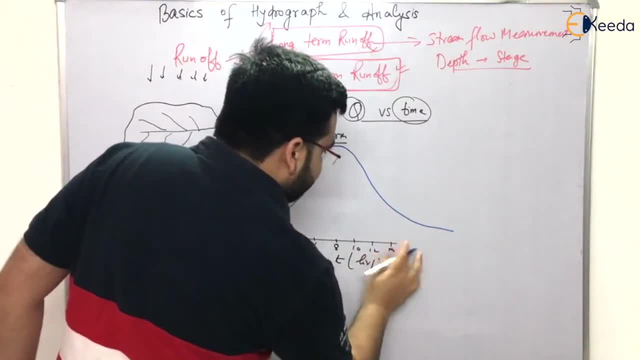 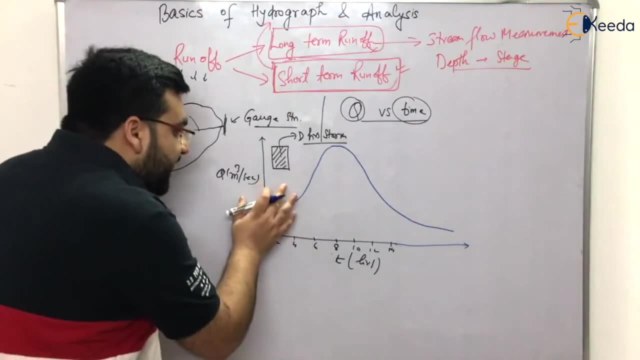 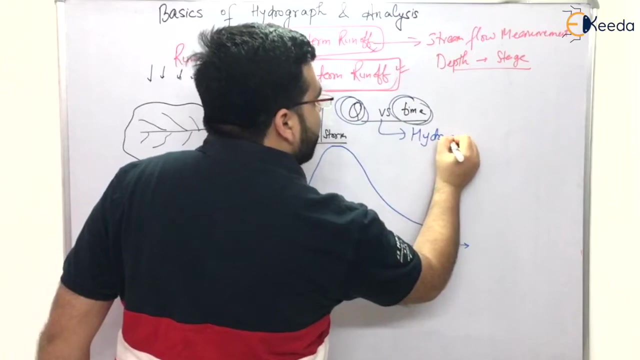 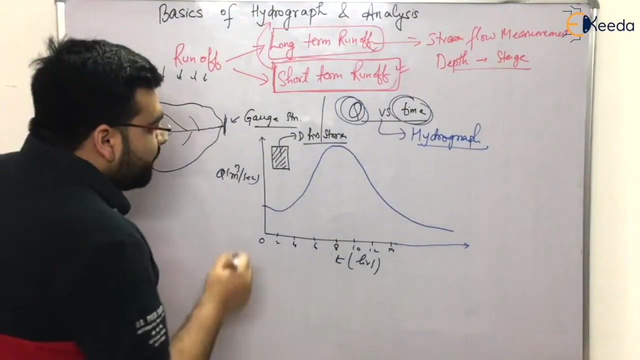 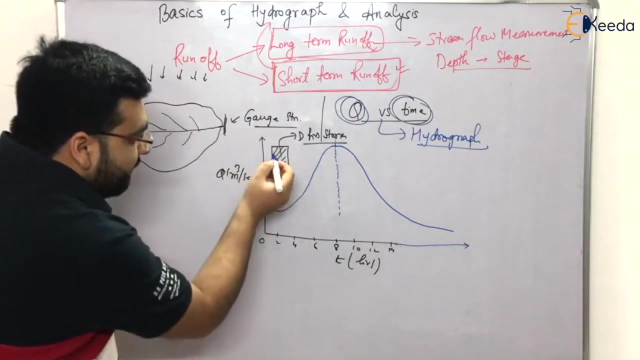 it will again recede like this. let me draw the graph like so. this graph again, I am repeating: this graph between discharge and time is known as hydrograph. right Now, the time, the distance between the peak right. obviously there is lag right. for example, the discharge, the precipitation was happening between 2 to 4 hours, but we are observing. 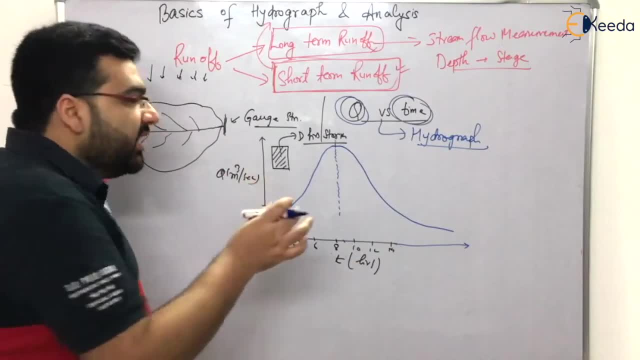 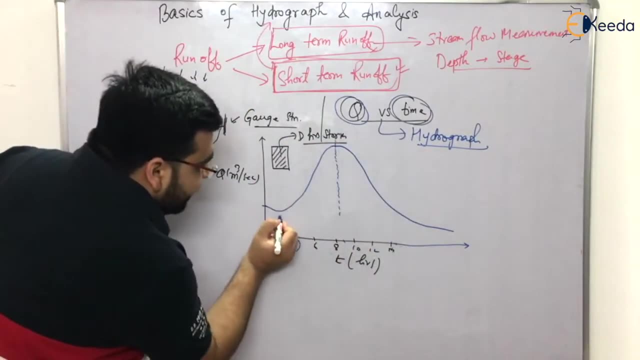 peak at, let us say, 8.5 hours. obviously there is a lag, that is known as a time lag clear. so this hydrograph has few. you can say parts right. So let us say: this is your first part. let us say A- clear, this is your. you can say B. 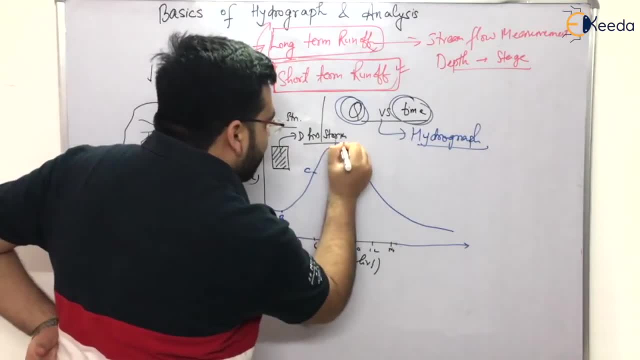 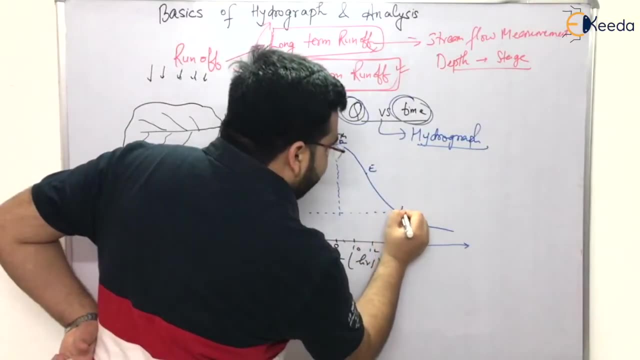 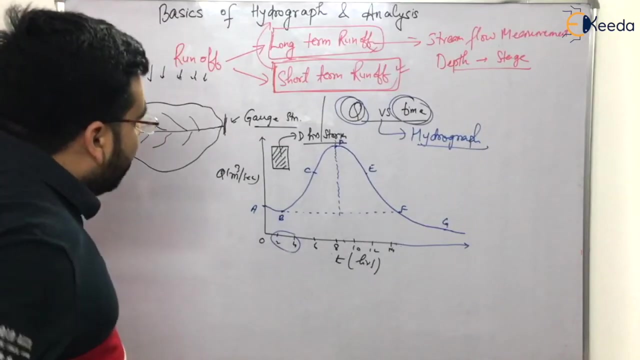 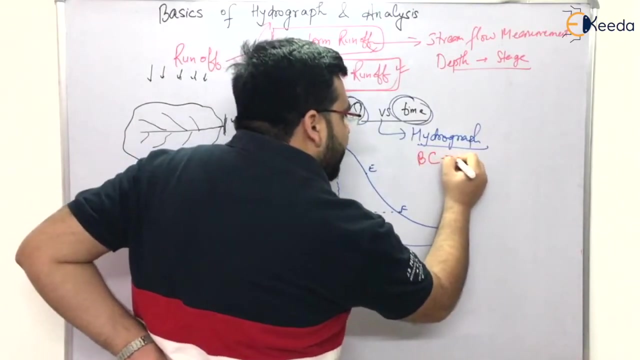 part. this is your, let us say- C part, this is your D part, this is your E part, this is your F part and this is your G part. clear, so it has a few parts. right Now, this part, that is, B to C part, this part, let me write it here: the B to C part is going. 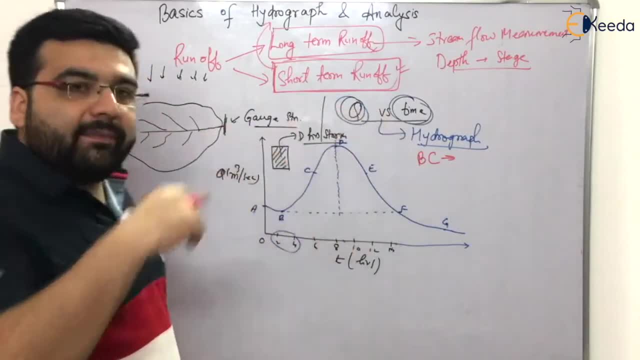 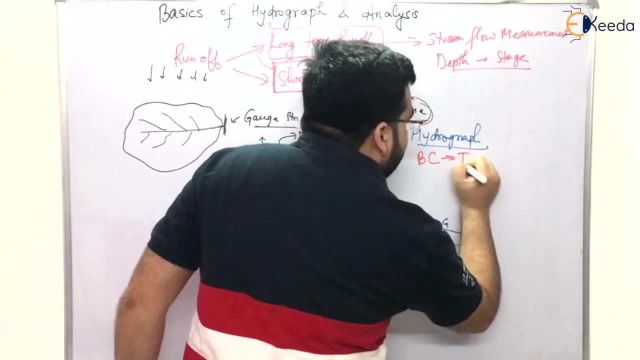 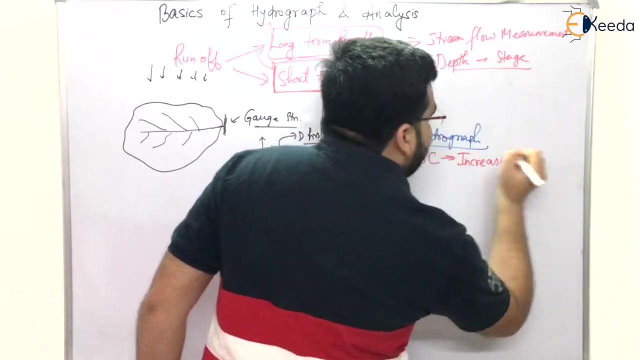 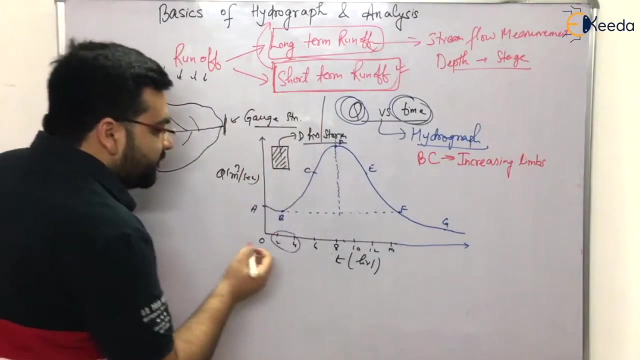 to be known as the. you can say leading limb right, leading limb right, or you can say succeeding limb right, or you can say it is increasing limb, increasing limb. if you go to different books, so different names have been given to this part: right, increasing limb, succeeding limb, right, or other names also. so this part B to C is increasing actually. so this is known. 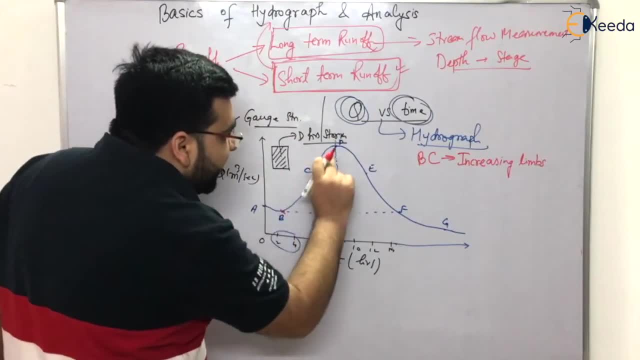 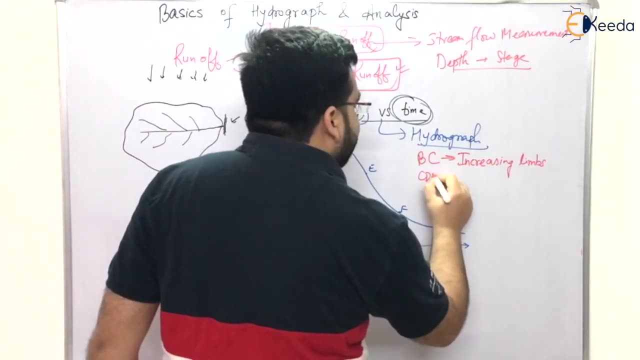 as the increasing limb right. This part- C D, E- is known as the crest right. so you can say that the this part that is C D, E, is known as the crest crest of the hydrograph right. this E to F part in most of the books. 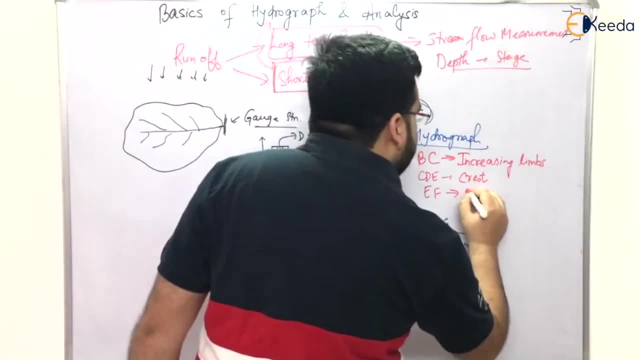 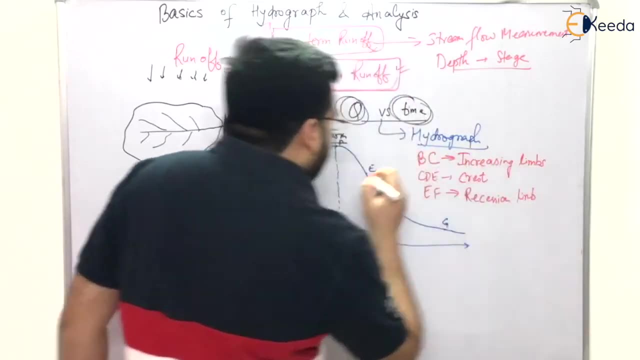 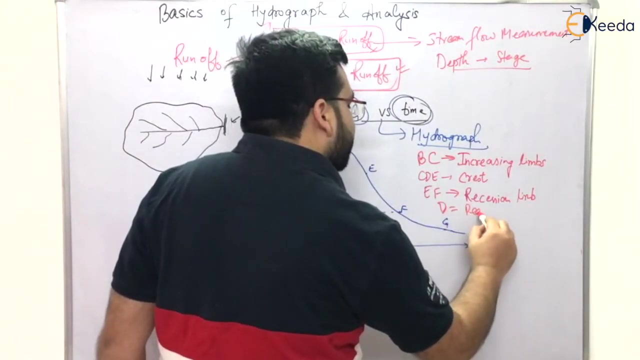 the name is given as recession limb right. this E to F part is known as the recession limb. recession means decreasing right, recession limb And this D. this point is called the recession limb right is the peak right. point D is the peak discharge. you can see peak discharge. 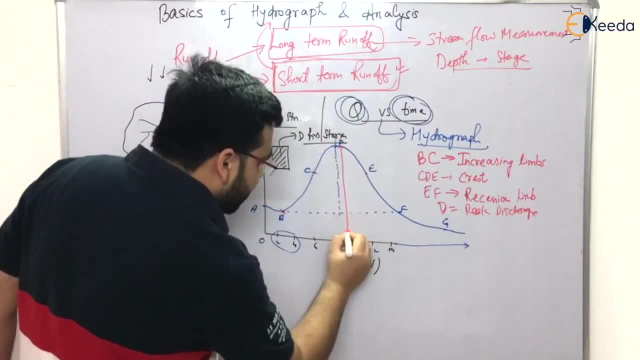 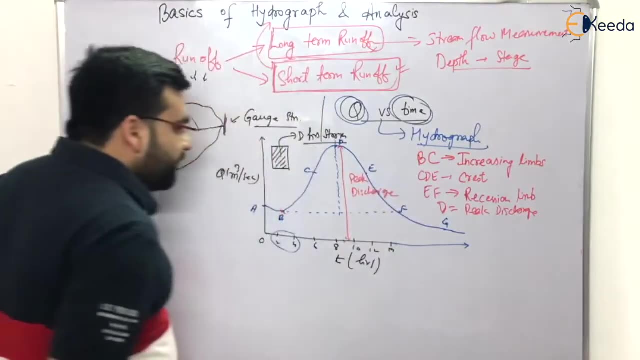 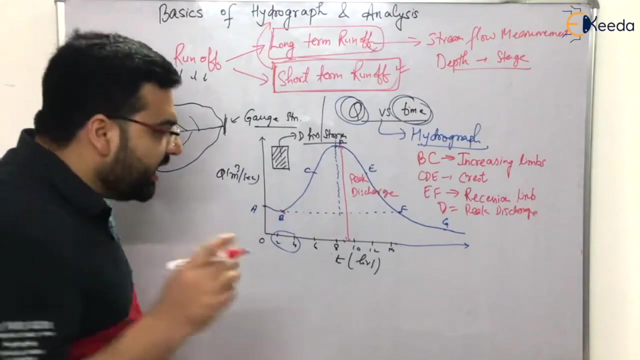 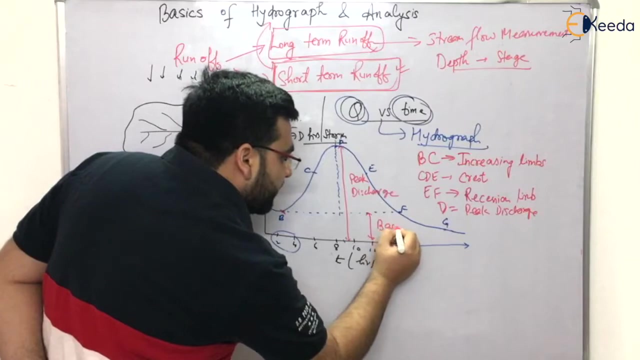 because if you measure from this point to this, it is a peak discharge, peak discharge. now, this flow. I told you that that before the storm has actually happened, there was some flow in the stream, right? so this flow, if I draw a straight line, this flow is known as the base, base, base. this flow is known as the. 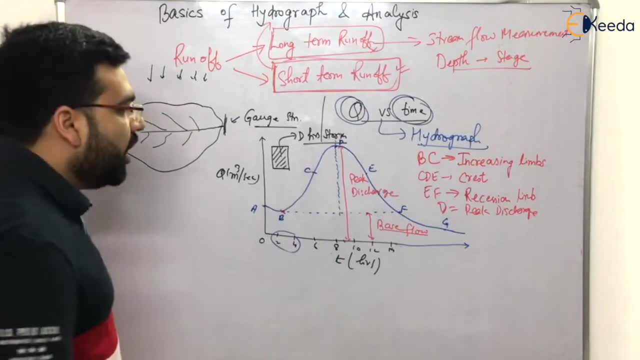 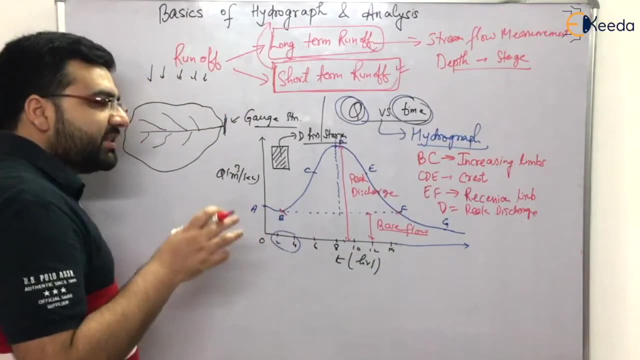 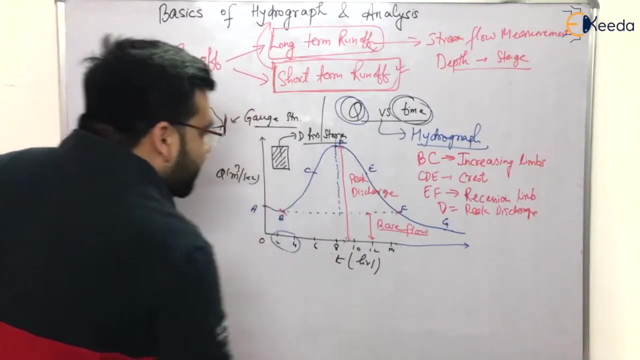 base flow. so these are a few parts of hydrograph now if you go to a different books, so this distance is also given, because it is very difficult to measure this. you can say this time interval, it is very difficult. also, you can say that this distance is also given in some books. so the distance is actually. so you 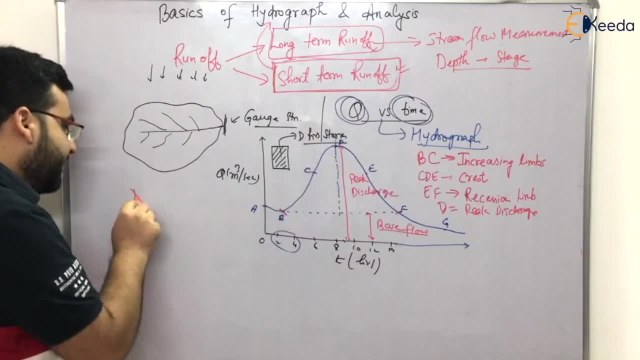 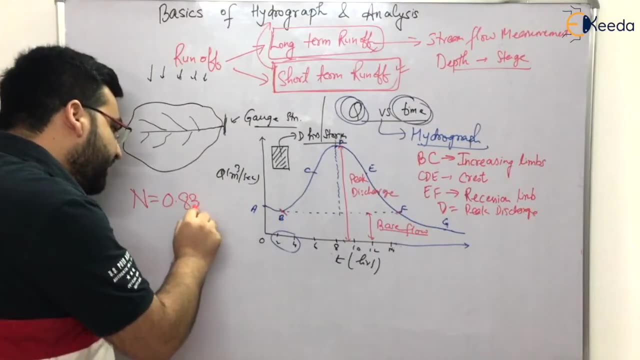 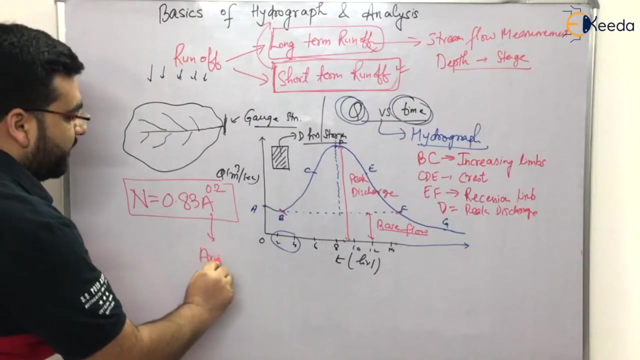 can. let us say that this distance is given by n right, so n. in a lot of books it is given as zero point. n is given as 0.83. a to the power, 0.2, where a is the area of catchment, area of. 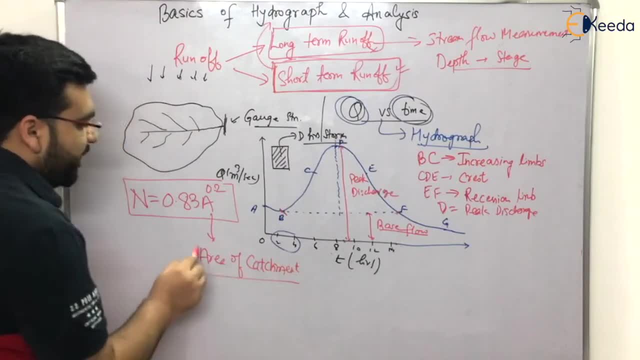 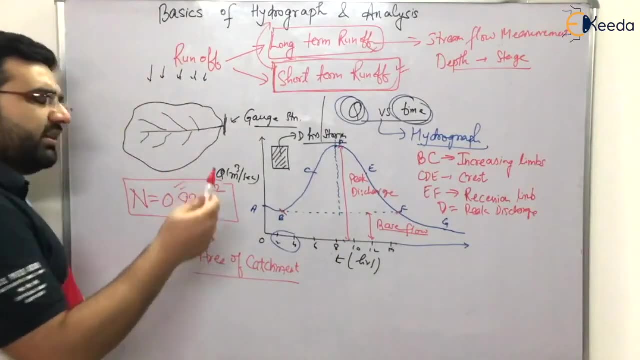 catchment. so in many books this value of n is also given, but that is not required for gate perspective. this value is not required, actually, right. even: if you want to learn it, learn it well and good. if you don't want to learn it, don't learn it, right. so because this, these types of 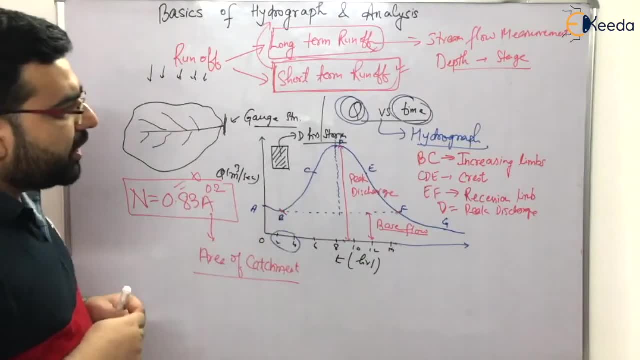 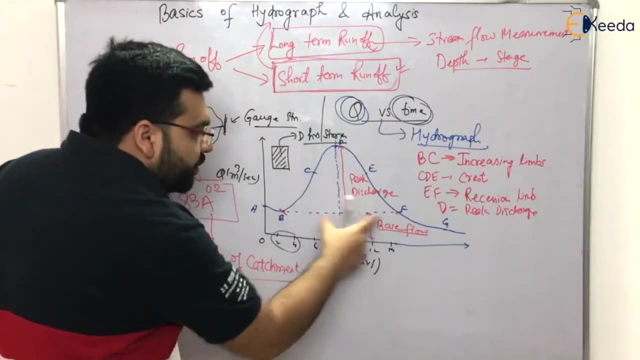 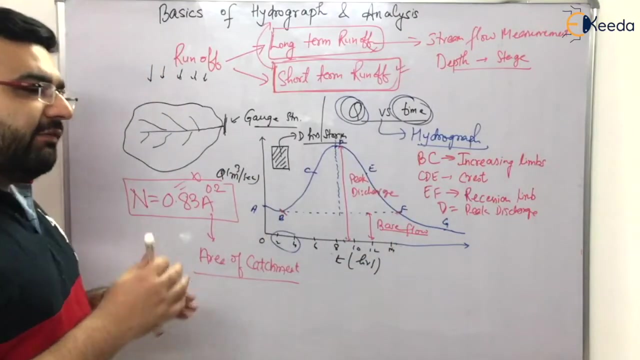 numericals in which this value is used are basically coming in your ESC mains examination. but as far as the gate point of view is concerned, this formula is not important, but you should know then how to remind this. you can say the time from B to F, so this is known as the base flow. base flow means the flow in the stream. 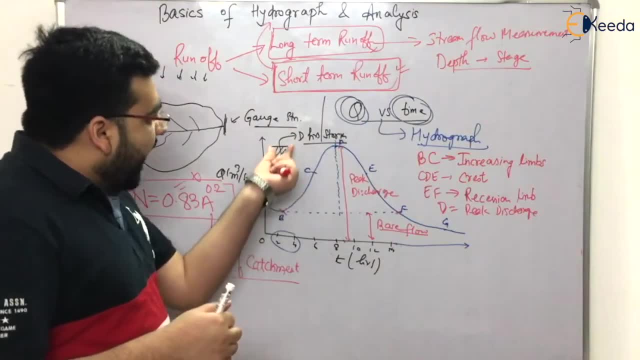 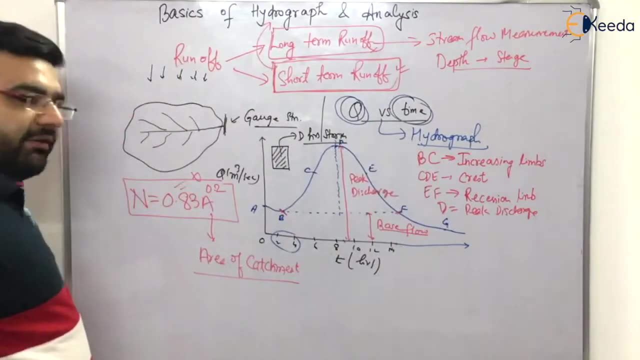 which was which was earlier to the the happening of this storm. that is known as the base flow. so I hope that you have understood the parts of the hydrograph now. there are a few factors on which the shape of the hydrograph will depend. there are a few. 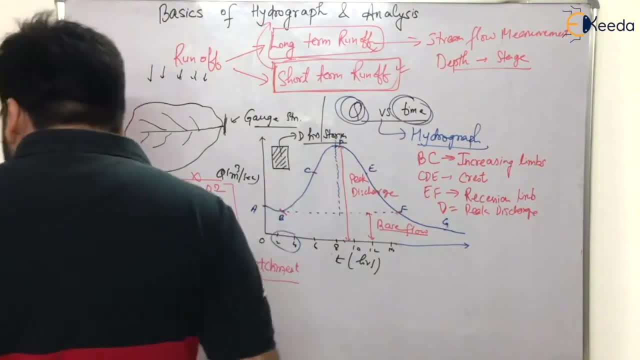 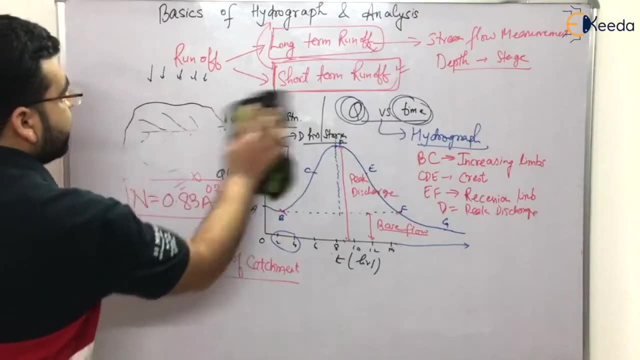 factors. so let us now study those factors on which the hydrograph will depend right. so now let me rub this and let me tell you about a few factors on which the hydrograph will depend right. so let me rub this. I hope you have got it: the hydrograph right now. 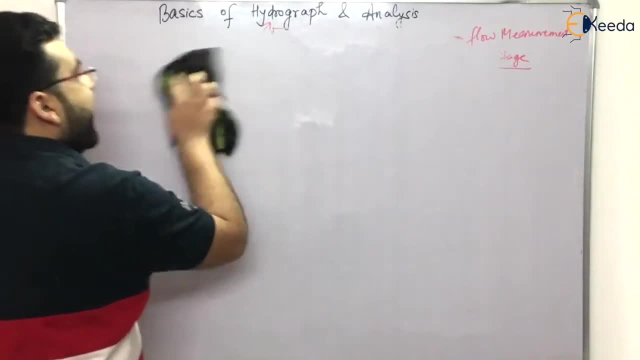 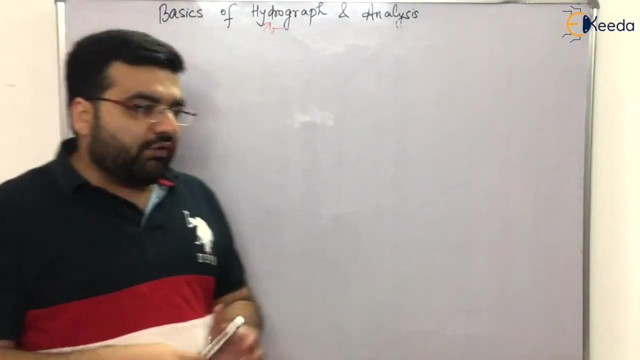 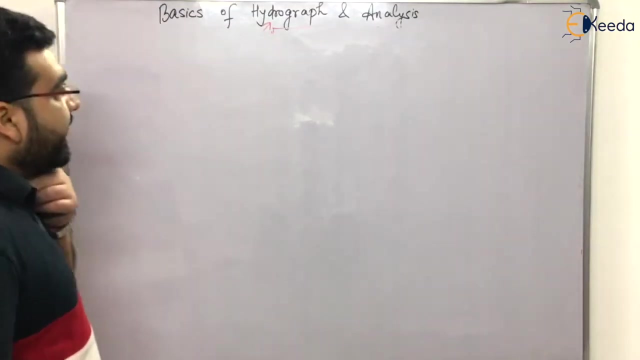 there are a few factors on which the hydrograph it actually depends. so if somebody asks you, what is your, what is the hydrograph, you will see that over a particular catchment area. if you draw a graph between this chart versus time, the graph is known as a hydrograph. simple, right, okay. now hydrograph depends upon a. 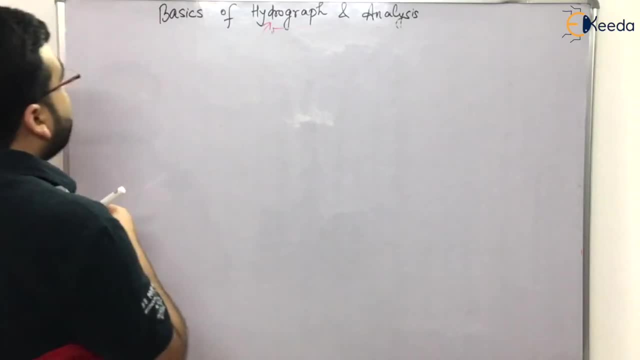 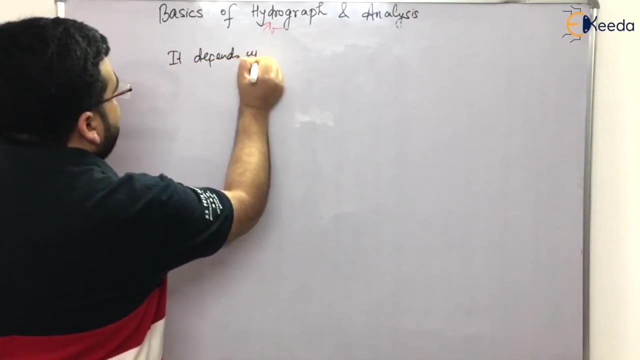 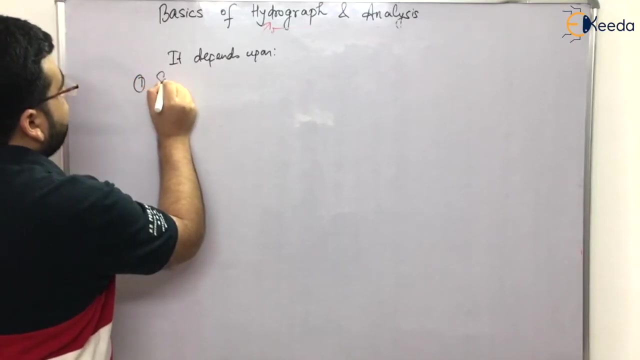 few factors, right? so first of all, let me write down it depends upon. it depends on because questions can be asked, theoretical questions, from this topic which I have explained just now, right? the first is size of the basin or the catchment size before size. first of all, let me tell you about shape right before. 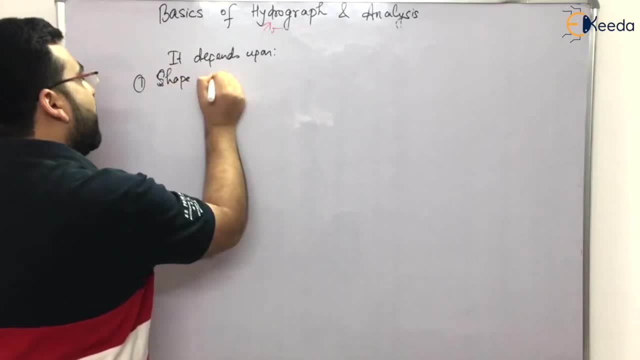 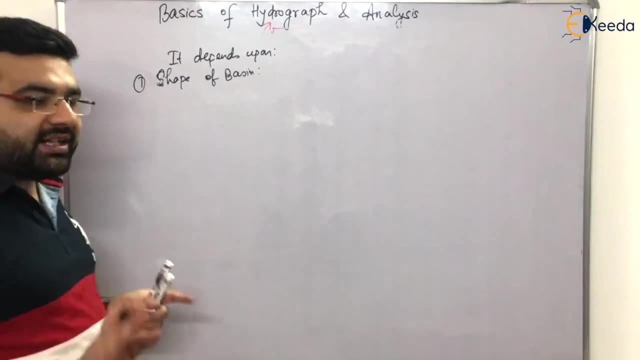 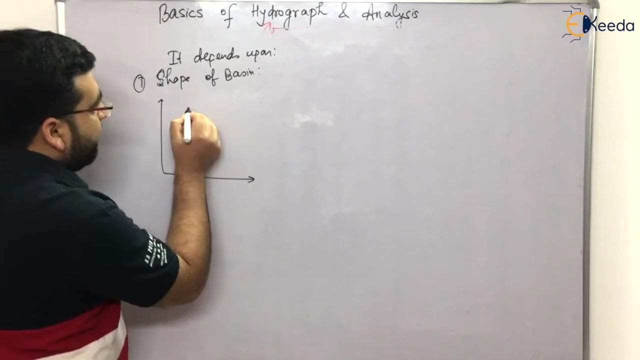 size. let me tell you what shape- shape of basin- and this question, which I am going to just tell you just now, it has been asked in many examinations, not just examinations but other examinations. okay, so if you have a shape like this, let us say this is your hydrograph. if the shape of the basin is like this, 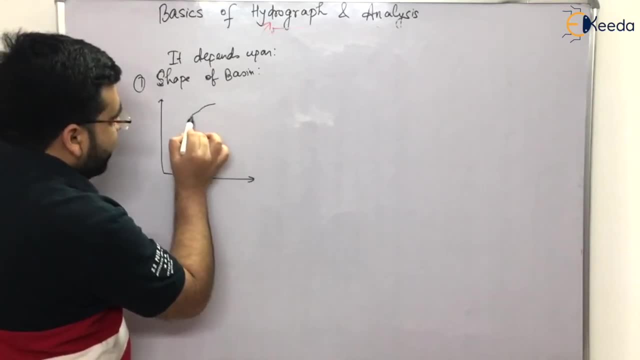 initially it is, you can say, thinner and then you have a large area. if you have a shape of a basin like this and the gorge station is somewhere here, this is the main stream, these are the tributaries, right. so the graph of the hydrograph and 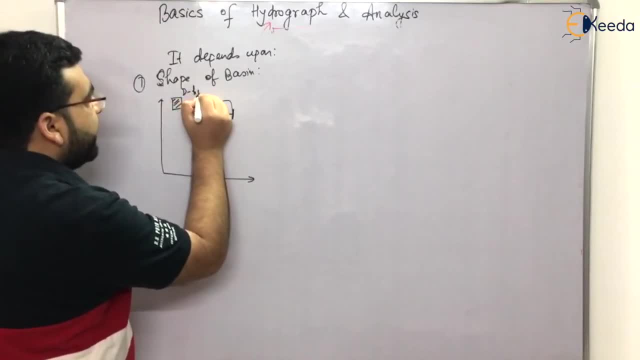 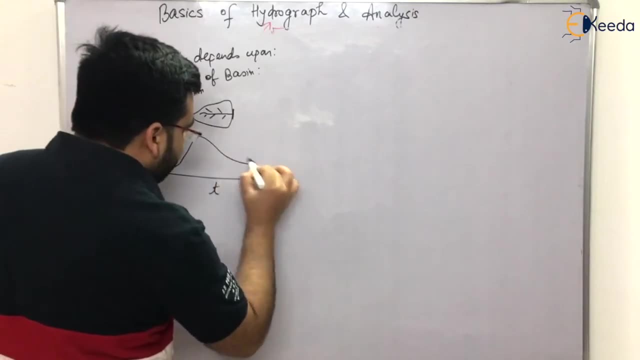 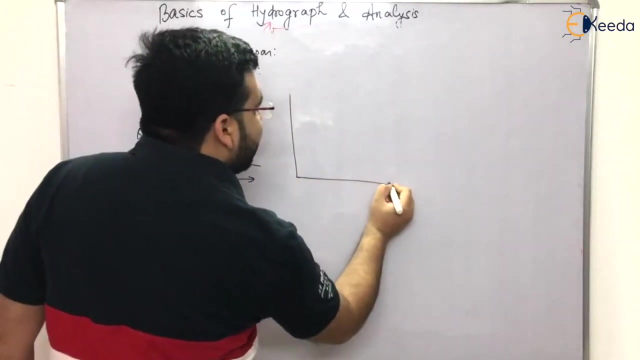 the storm has fallen over a period of time D, DR storm. this is your Q, this is your time T. so the shape of the hydrograph will be like this: that initially it is broad, but at the gorge station is narrow. right there's a lot of station. this is the main stream. these are attributive things, right, and 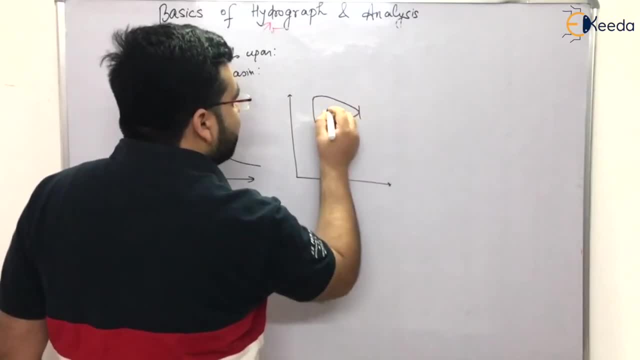 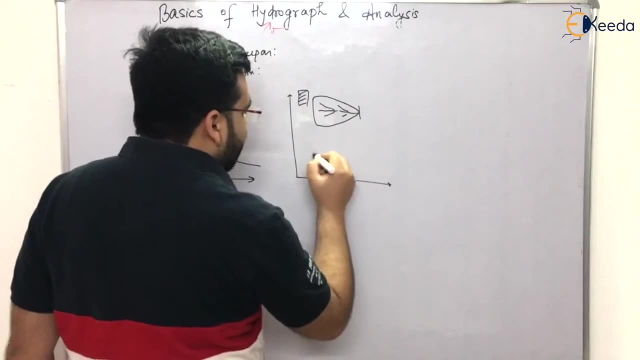 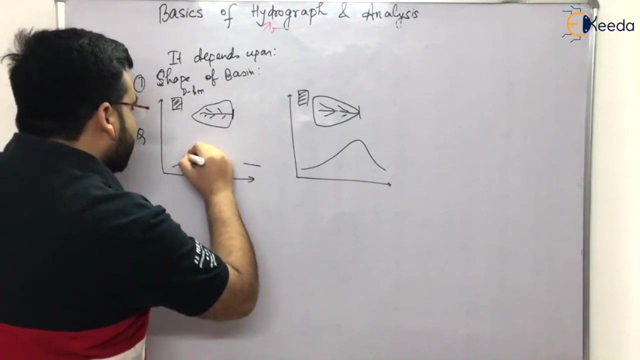 your storm has happened, baby asked. oh so the shape of the gra until earth will be like this for this part? right, then we draw it more precisely so it will be more precisely skewed to the left, it skewed to the right and here. so now sun day, 쇼 can see, but now sun is. this composition is beyond this convention to 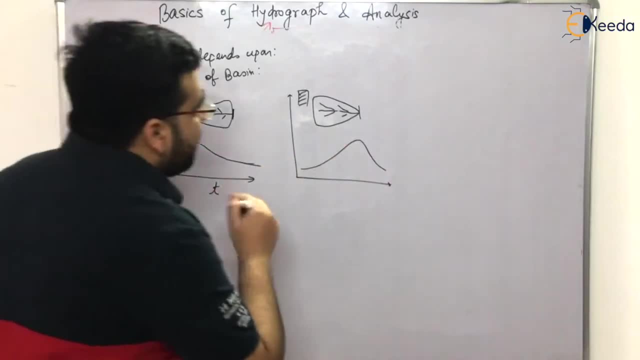 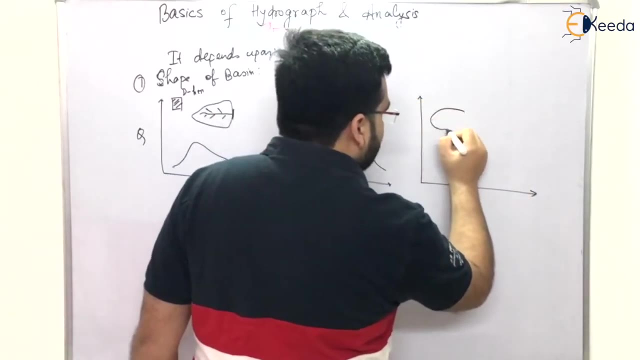 be based on this for Familie system. okay, like received to appears where it will be the right right. but if the shape of the basin is like this, if the shape of the basin is like this, is like this: this is the stream, these are the tributaries, is 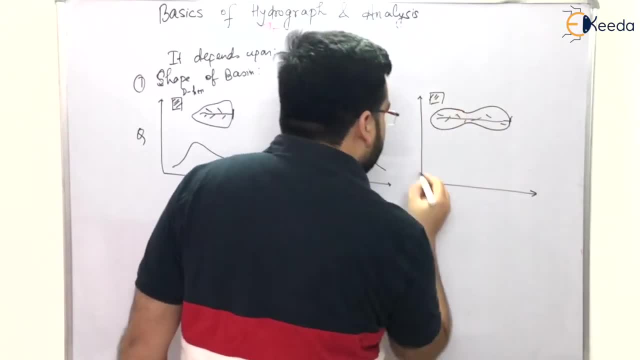 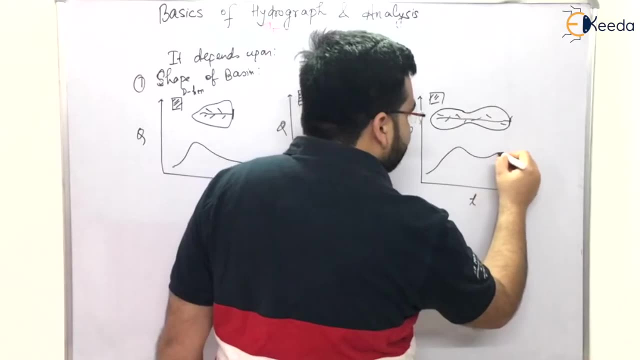 the God station and storm has happened, or this period of time. this is Q, this is T. this is Q, this is T. right, the shape of the hydrograph is like this: we have two peaks. this is the shape of the hydrograph. okay, so I hope that you have. 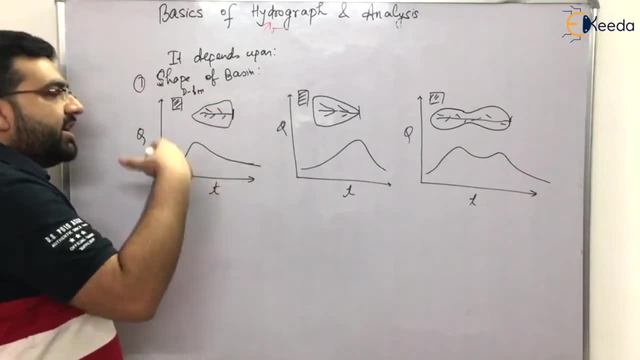 understood that how the shape of the basin or catchment- it you can say it- influences the shape of the hydrograph right. so if you have a shape of a catchment like this, you have a hydrograph like this which is, you can say, skewed on the left. if you have a shape of the catchment like this, you have a graph. 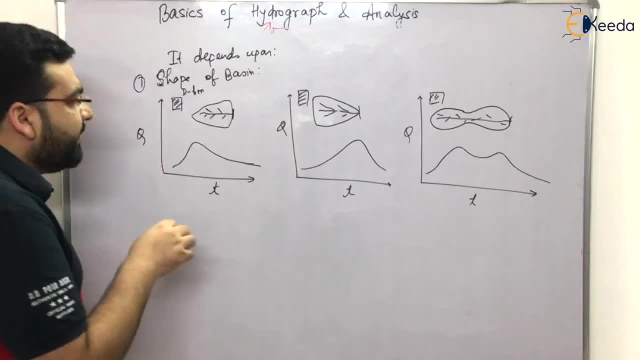 hydrograph like this skewed on the right right now, why it is actually happening? because you can say: let us see that the rain is falling on this catchment area. let us say there is a reason also. let us say that the rain is falling on this catchment area, so this is narrower right. 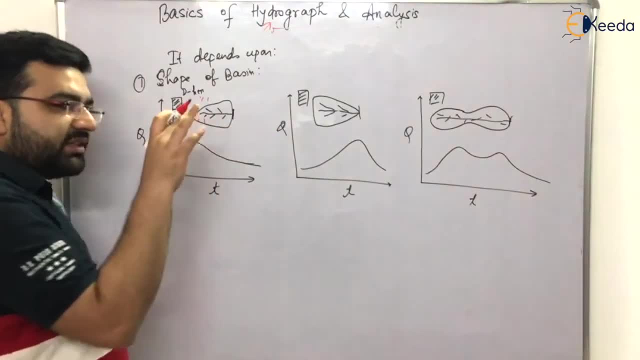 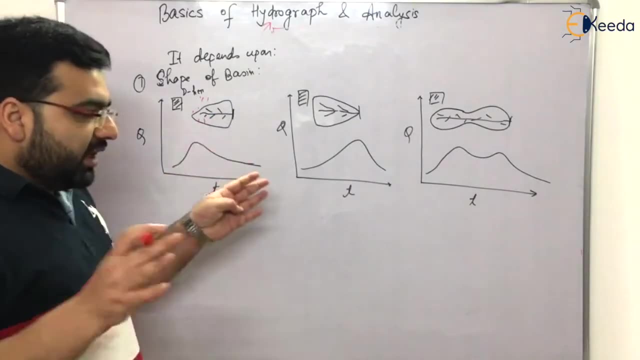 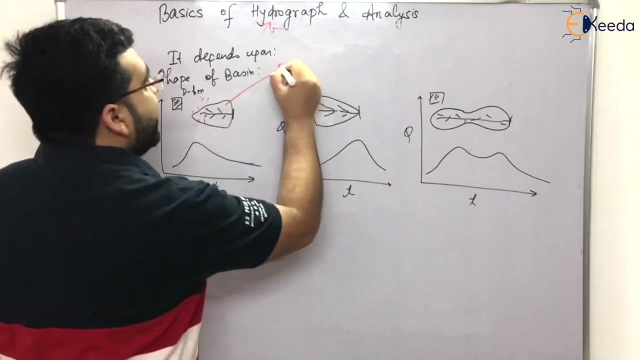 it is narrow, it means the area of the catchment. this is, you can say, small. so the time interval for attaining the peak discharge will be very small because you can say a lot of water will be coming. you can say instantaneously because it, for example, let me draw it bigger, let us say this is bigger. 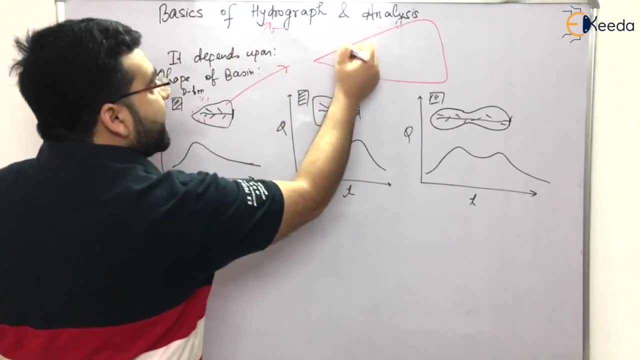 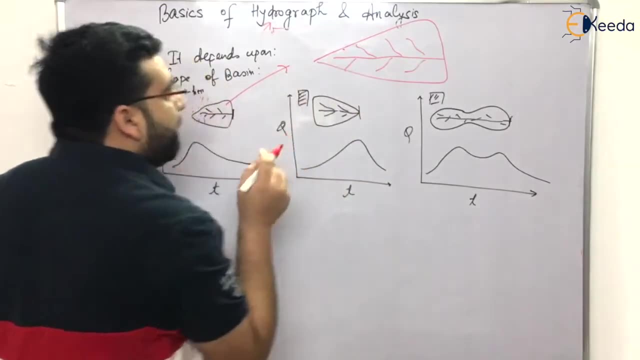 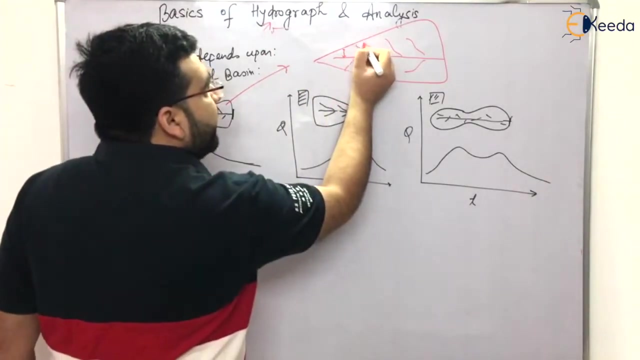 this is bigger, right, so some rain has fallen on this area. there is the main stream. these are the tribute trees, right? so this particular particular rainfall will take a very small time to reach this stream. similarly, the rain which has fallen on this area it will take a very small time to reach here. very small time, very small. 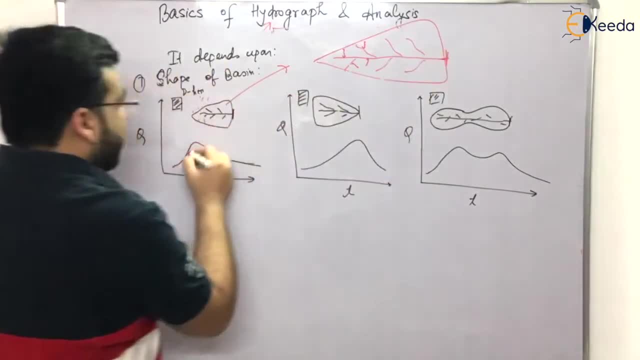 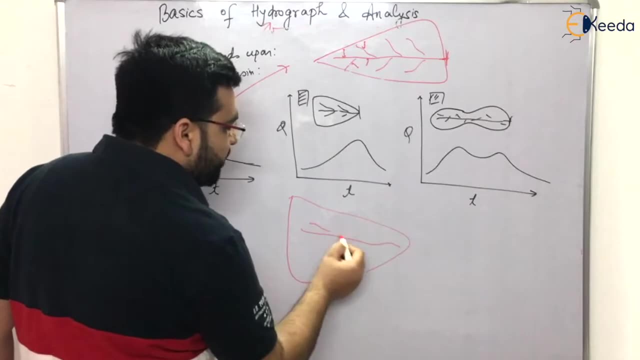 time, very small time, and hence in a very small time you will attain a peak discharge. but as far as the second is concerned, let us say you have a very broad area here. there is the main stream, these are the tribute trees, and the gorge station is here. if suppose that some rain falls on this at this point, so it. 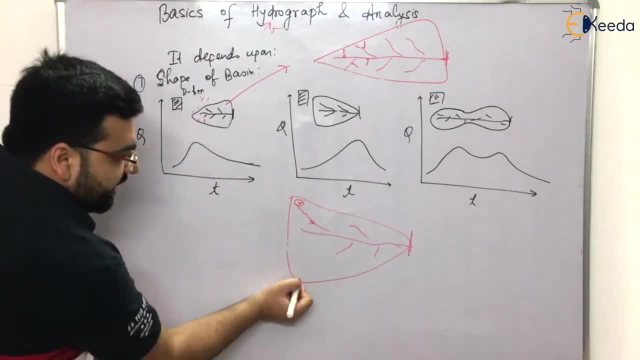 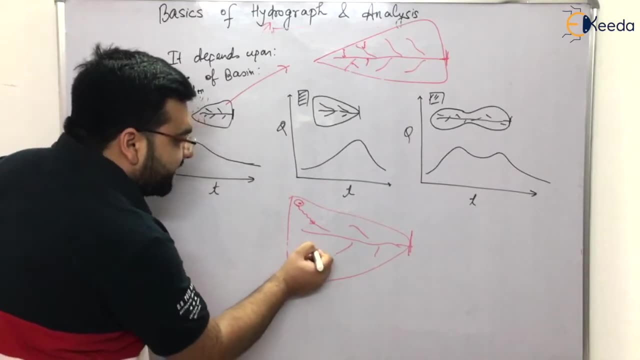 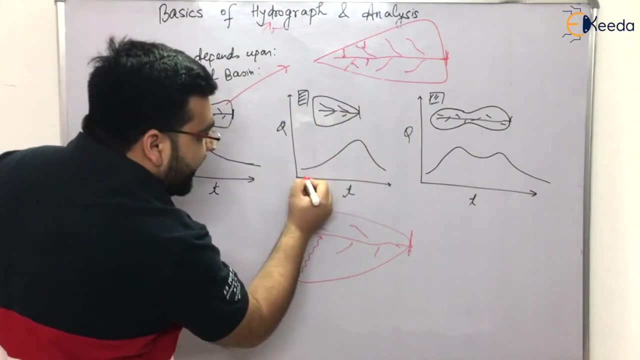 will take a lot of time to reach the stream. similarly, if this some rain has fallen on, precipitation has come to this particular area, it will take a lot of time to reach the stream. so hence it will be the chosen. it is a, you can say, skewed on the right side, because it will take a lot of time for to attain a peak. 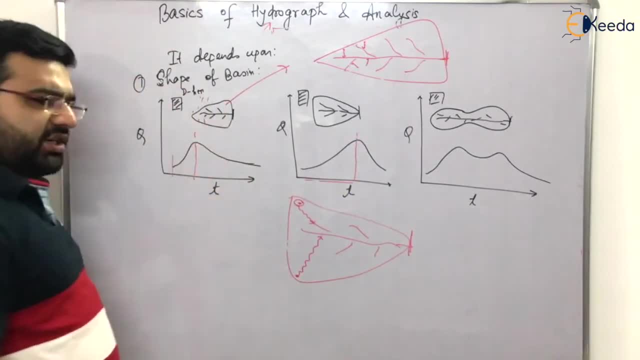 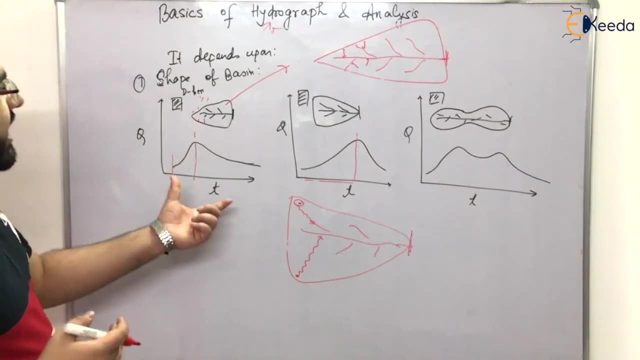 discharge, and it will take a very small time to attain a peak discharge, simple yeah. now, after the shape of the basic, the second factor which is determining the, or which is influencing the hygrograph, is the size of the basin. so let us discuss about the size of the basin. 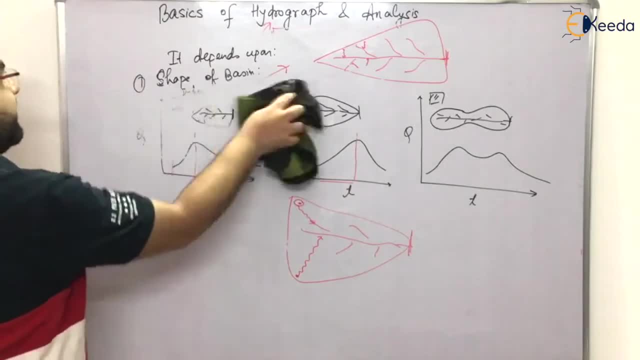 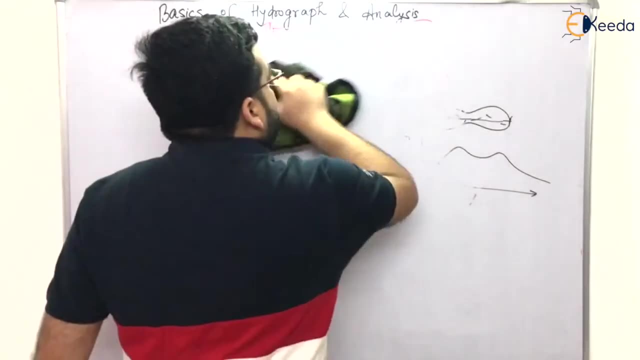 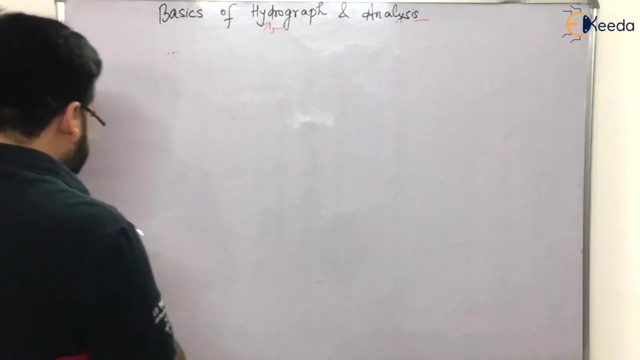 right. so after shape, I let you discuss about the size of the basin. let me look this right. the second factor is size of the basin. now, size of the basin also has the same influence which I have just told you, just explained you. so second one is number B is size of the basin. now, I'm not going to tell you, you tell me. 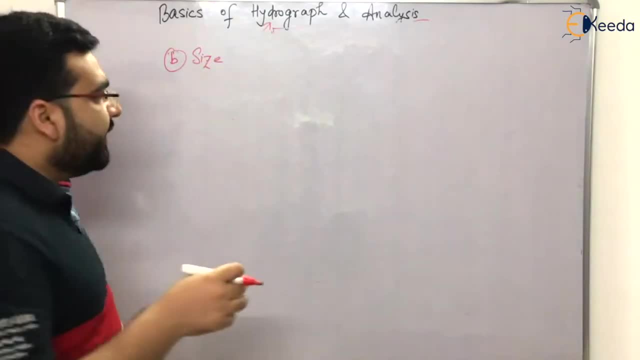 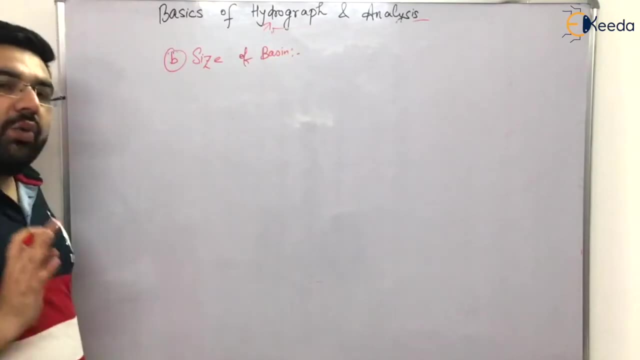 what do you think what will happen to the hydrograph if the size of the basin is very large? right, the size of the basin you tell me? just think and tell me. what do you think? what will happen to the hydrograph if you can say the size? 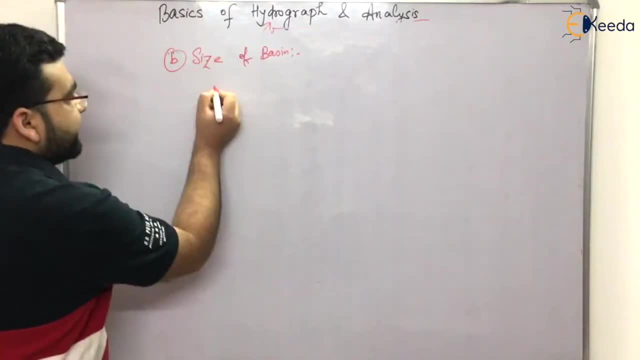 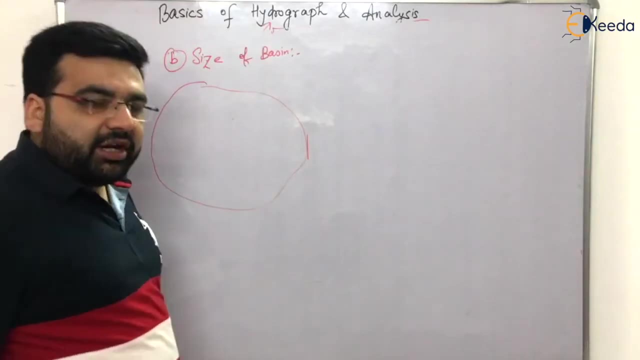 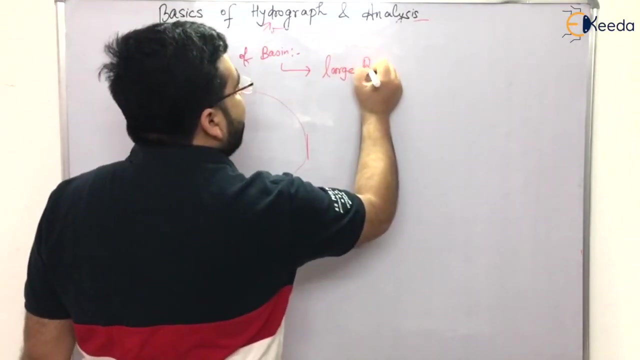 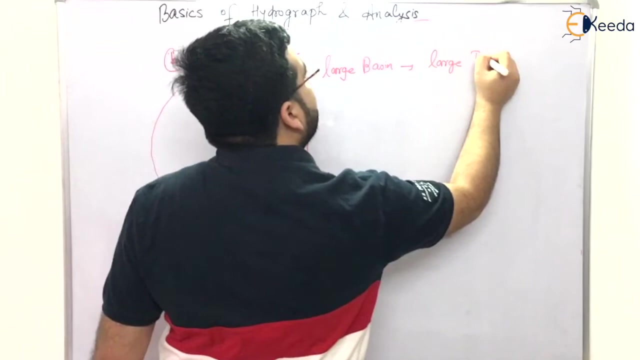 of the basin is very large. so it is just common sense that she, if the size of the basin is very large and you have a gorge station here, it will take a lot of time. it means that a timebase will be very high, right? so you can say that large basin, big thing, large time base. 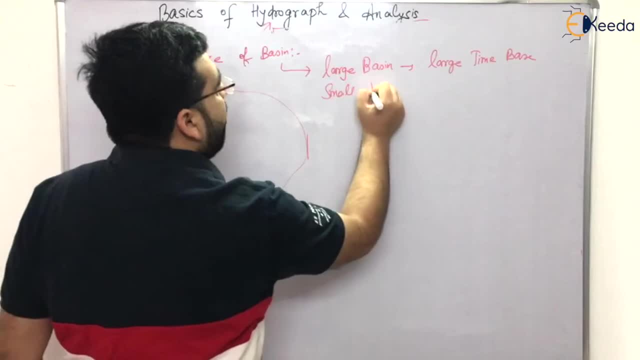 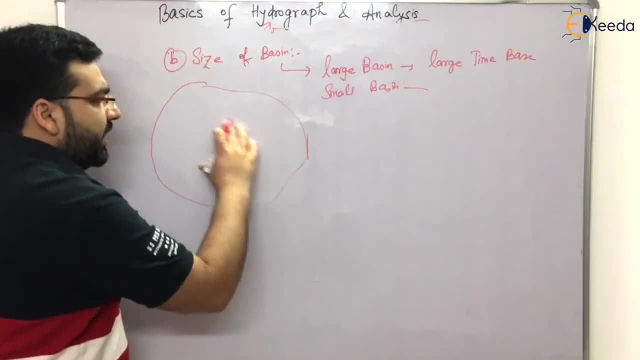 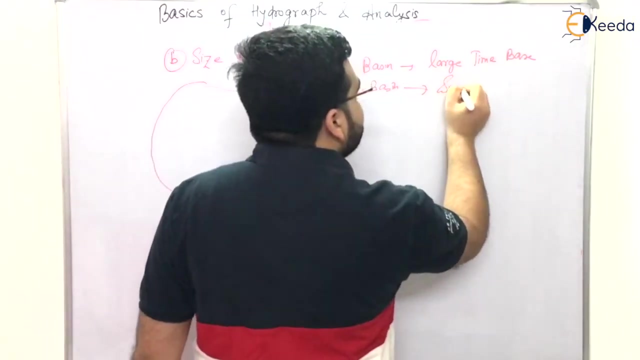 and small basin here. if it is this small basin, then the hydrograph will be of a very short duration. in a very short duration all the water will go to the main stream and hence it will be recorded by the gauge station right. small basin, so small time base. small time base you can write. 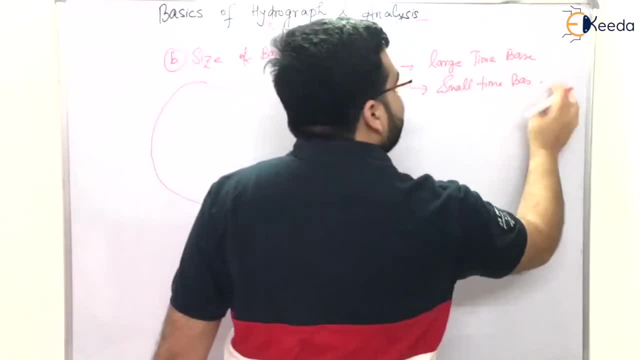 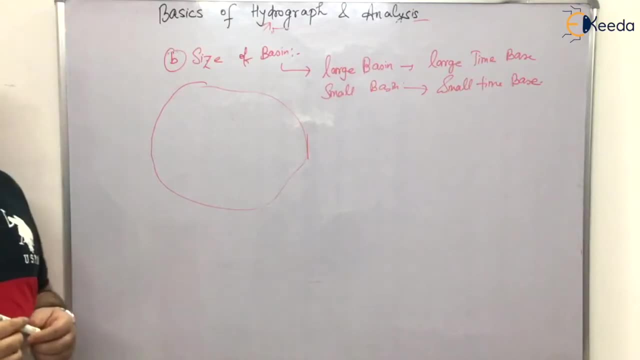 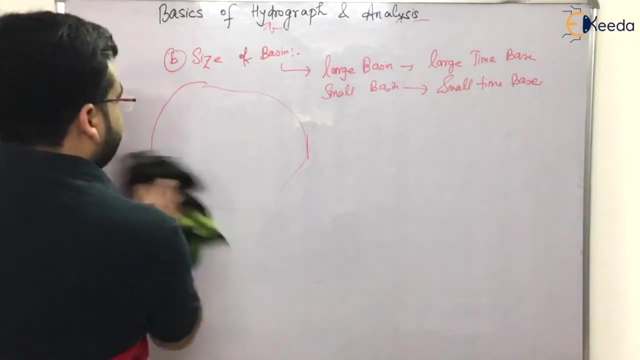 this in your own language. in your own words: small time base, right. but I have just told you the concept that what is the concept behind the size of the basin, right? so, after size of the basin, it also depends upon the slope of the basin also. so let me tell you what about the slope of the basin, right. so what? 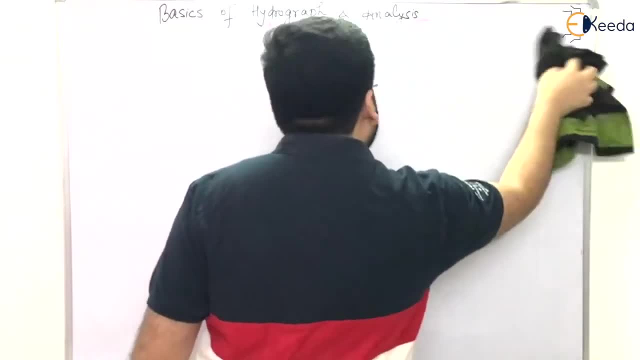 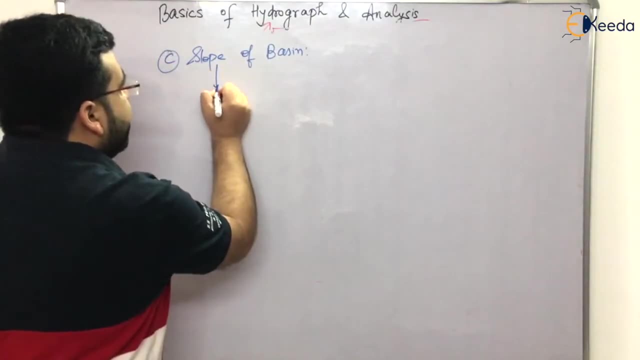 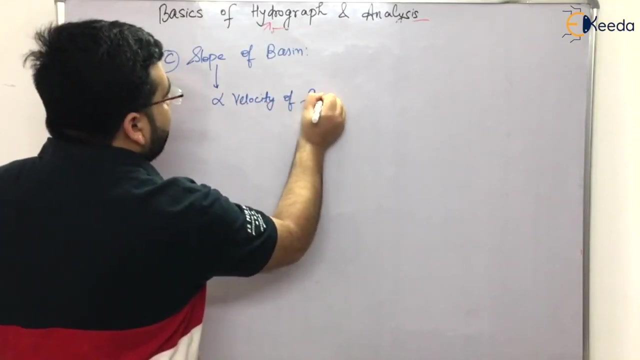 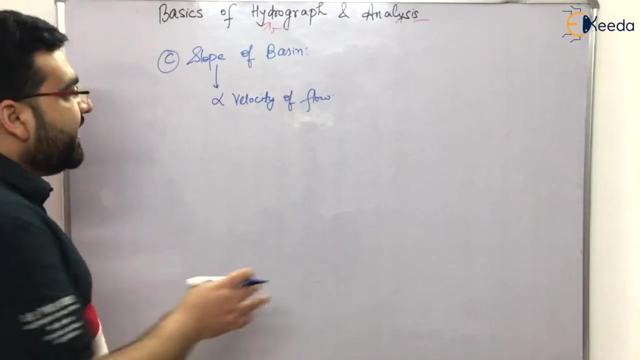 will happen if the slope of the basin is very high. so you know that slope, it directly influences the velocity, it directly influences the velocity of flow. velocity of flow: so slope of a basin directly influences the velocity of flow, but the slope of the basin will have larger impact. it will have larger impact on 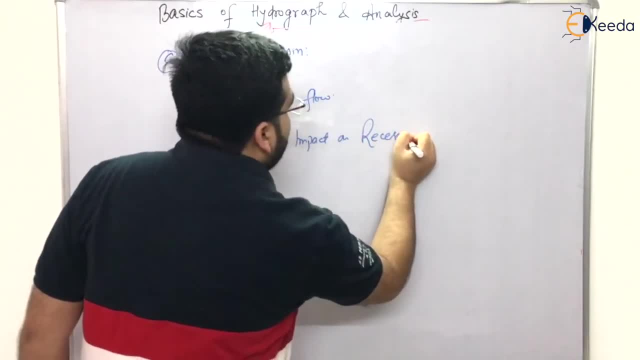 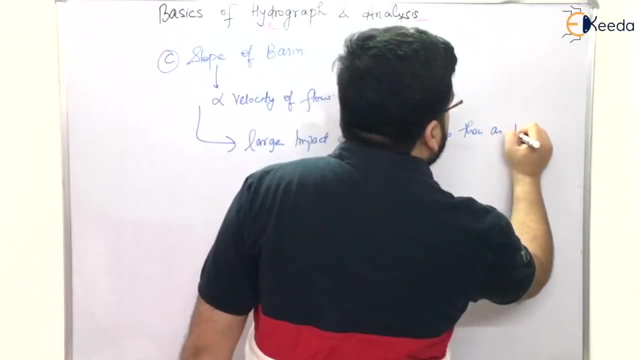 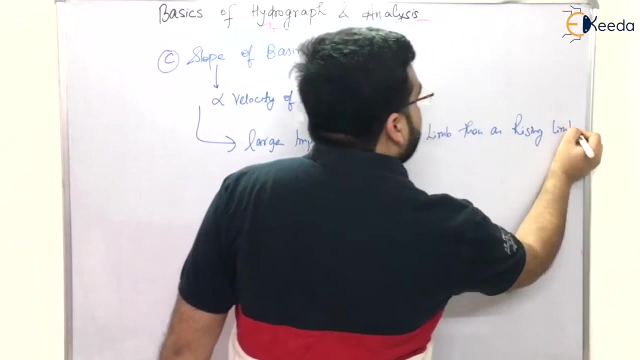 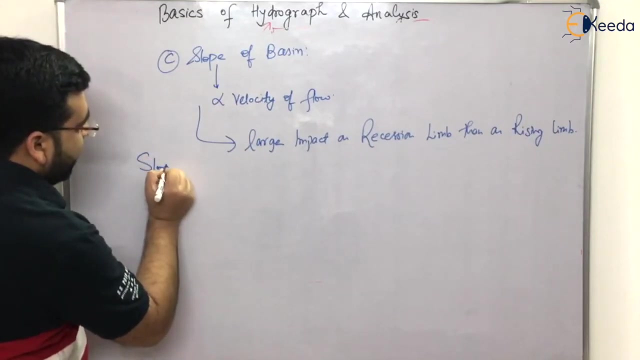 recession limb on recession limb, than on the rising limb, than on the rising limb, and that limb is also succeeding limb, also known as the rising limb. also right, the rising limb. okay, now what will happen if the slope of the basin is very high? if the slope is high, if slope is here, if soap is large, then if so bizarre they. 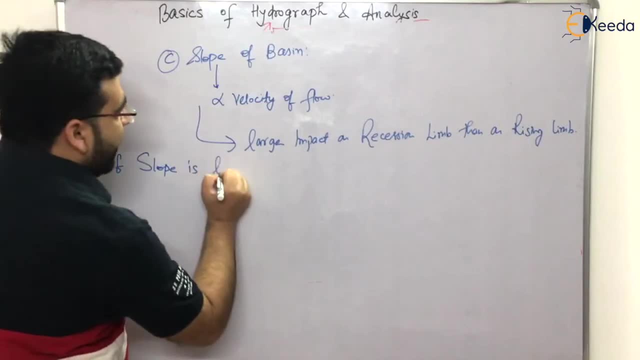 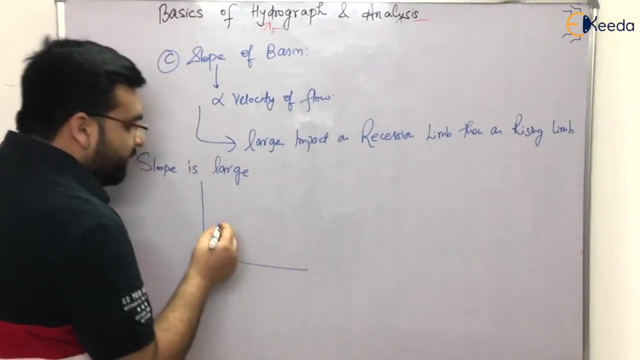 will think: then what will happen? this recession limb very small, or you can say the slope of the recession limb will be very high. so your height graph will be like this: it will be like this: so the recession limb will have a large. so it may be small, but if the slope of the recession limb may be very large, again I 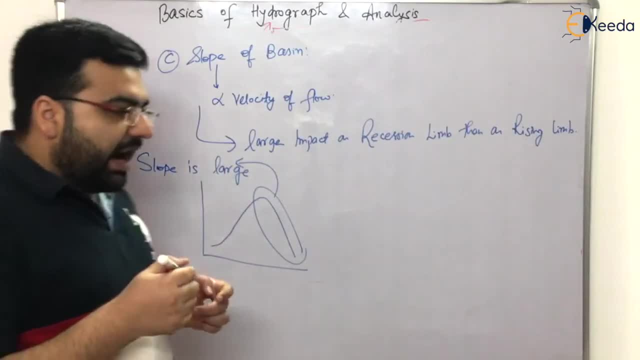 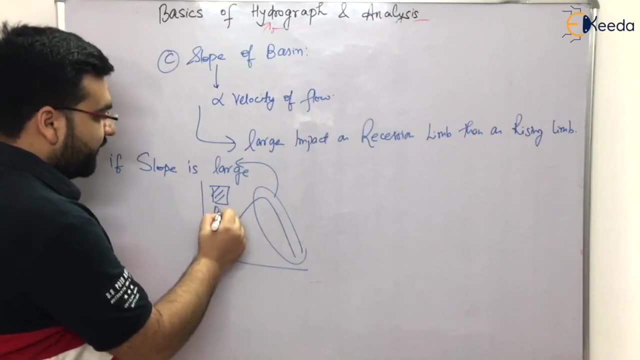 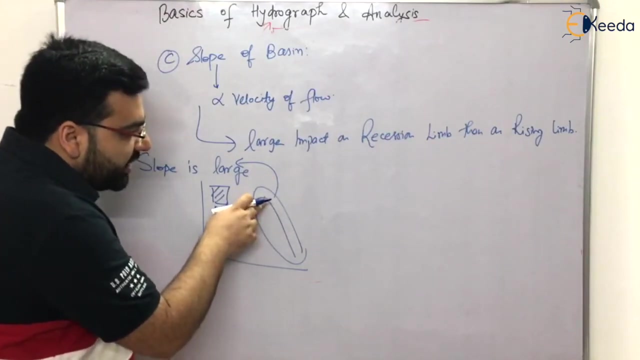 probably understand that now. what will then, if it will gap up, come door? Harvard means that after attaining the peak discharge when the storm, which was of D hours duration, now, when the storm is gone right now, after attaining the peak discharge, the discharge, it decreases rapidly if the slope of the basin is very large. that is the common sense now. 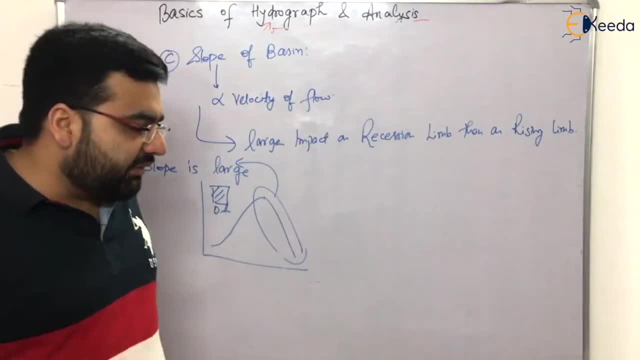 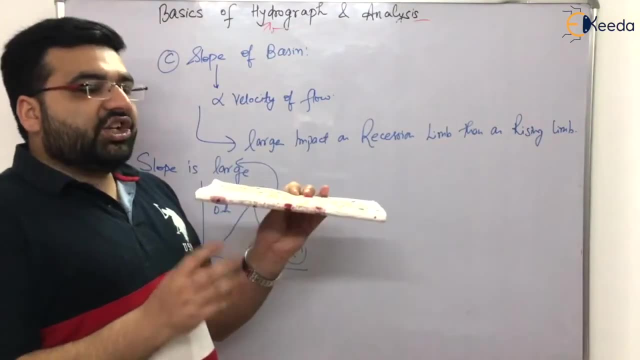 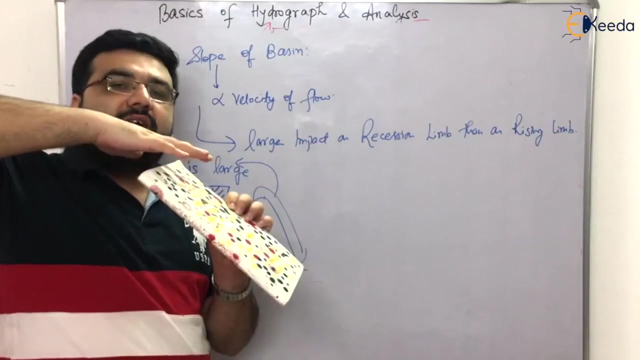 if the slope of the basin is very large. let me give you an example also. let us say: I have one notebook, right, this is my basin, this is my basin, right? so initially the slope was: let us say the slope is very large, very high basin slope if rainfall is happening on this. 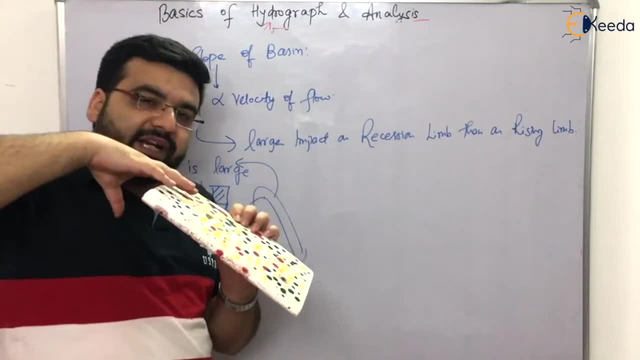 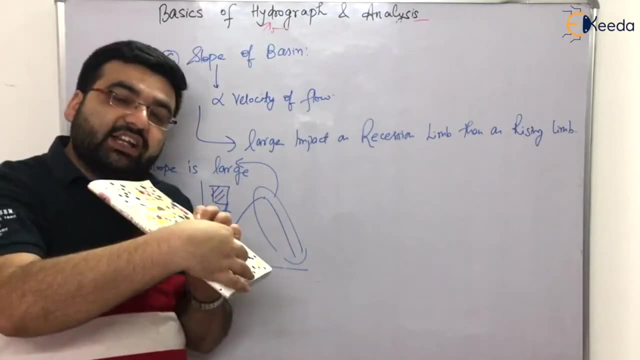 place. a storm has just arrived on this place and precipitation is there. so what will happen? this is the gorge station, so gorge station will record. you can say the discharge at a very short time and after the storm is gone. after it is gone, then whole of the water will. 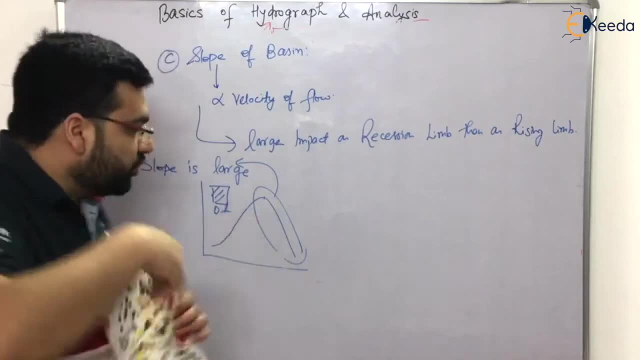 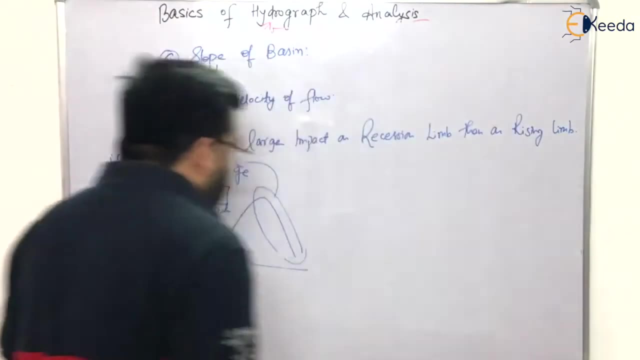 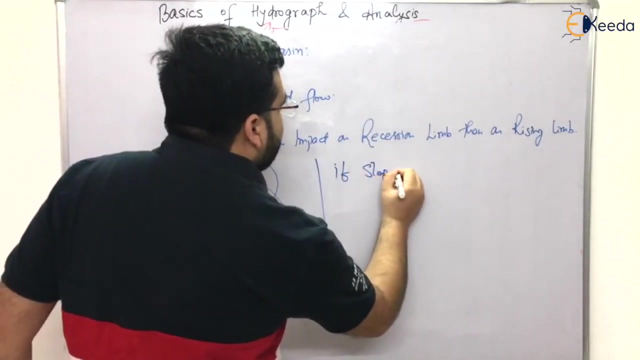 disappear rapidly, because if the slope is very high, so the recession limb will disappear or disappear very rapidly. on the other hand, if the slope of the basin is large, if the slope of the basin is less- now, if slope is less- then this recession limb will be larger. 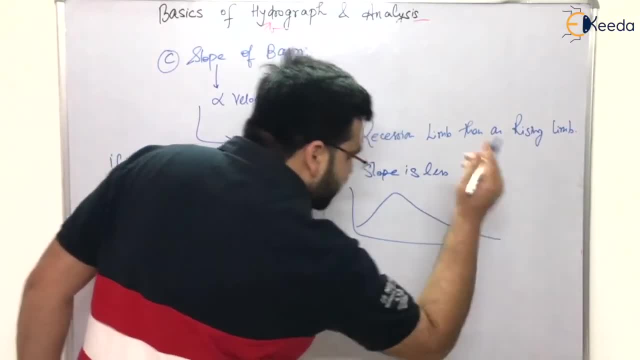 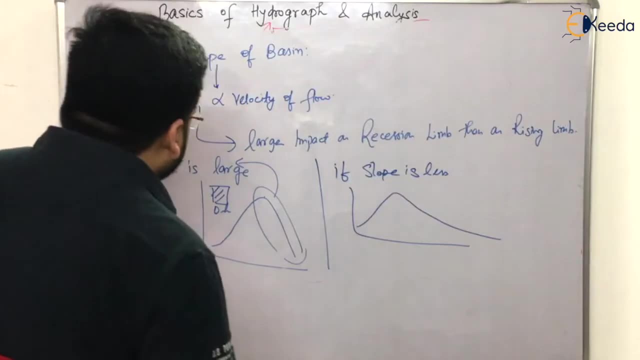 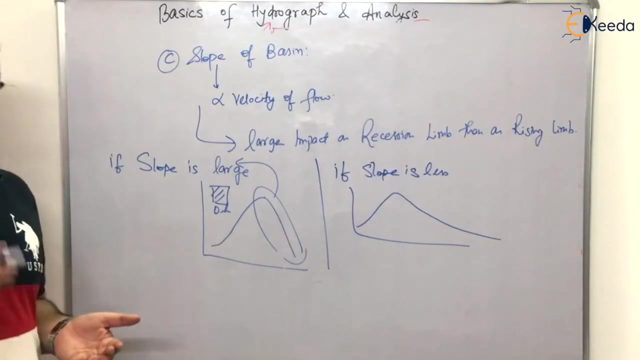 so it will be like this: discharge will then. it will be large like this: slowly, slowly, slowly it will disappear. ok, now, this is the third factor on which you can say the hydrograph it depends. now, the fourth factor is the drainage density. right, so now let me tell you about drainage density. 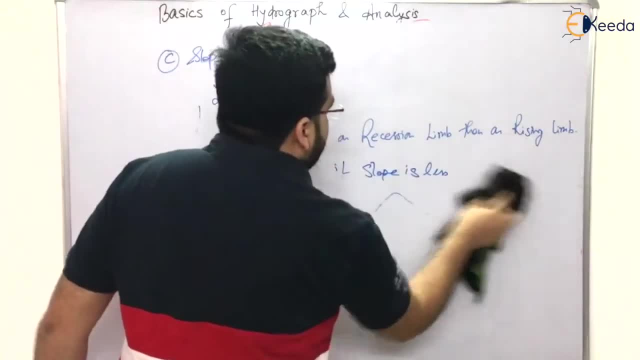 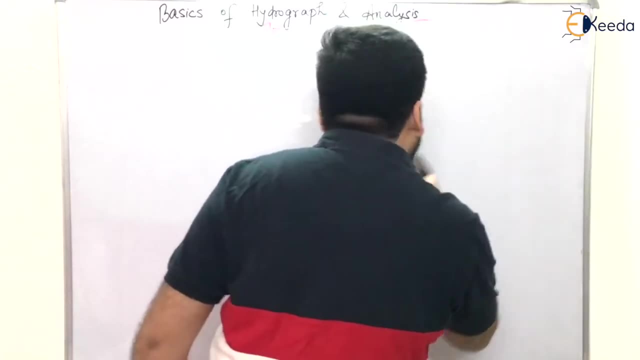 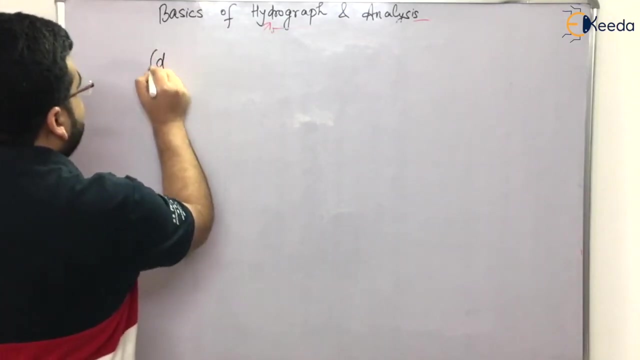 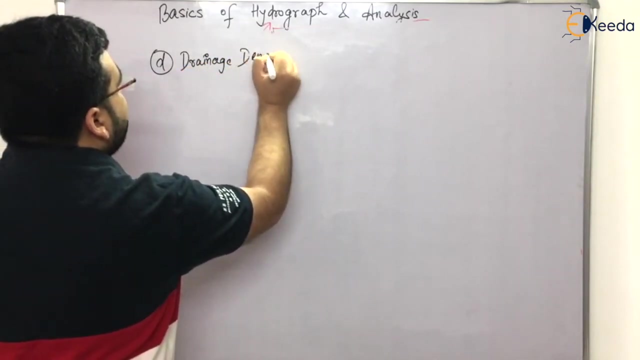 also now. what is drainage density? now, drainage density is the total length of the stream divided by the area of that particular catchment right. so what is drainage density? let me tell you now. fourth factor on which it depends is drainage density, drainage density. now, drainage density is the summation. 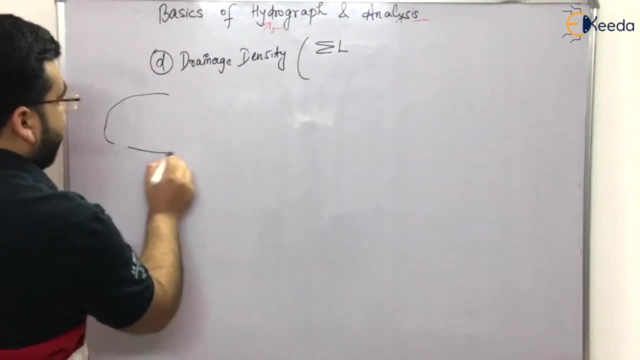 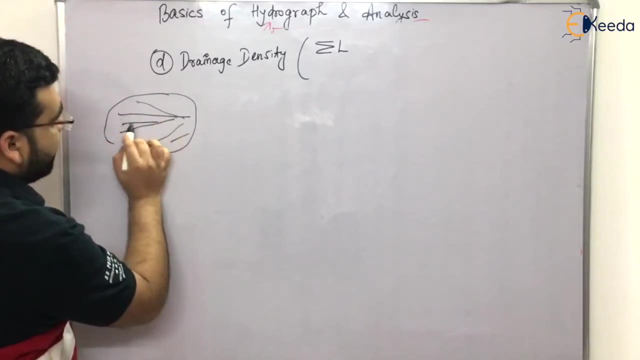 of total length of the stream. for example, this particular catchment area has a lot of streams, right, has a lot of stream. so summation of length length: one plus length, two plus length, three plus length, four, five, six, seven and so on, divided by the total area of catchment. 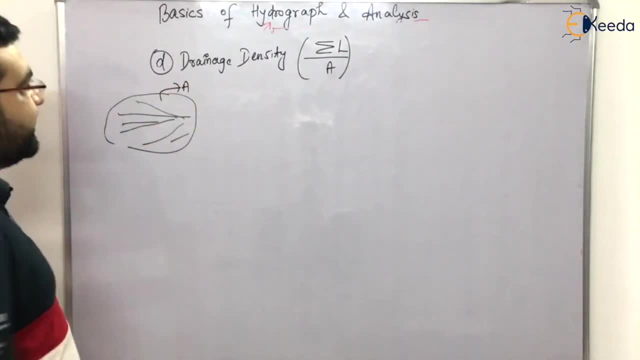 let us say the catchment area is a right. this is known as the drainage density. now you tell me, if the drainage density is very high, it means that there are lot of streams in the particular catchment area. so what will happen when a storm has happened, when rainfall precipitation? 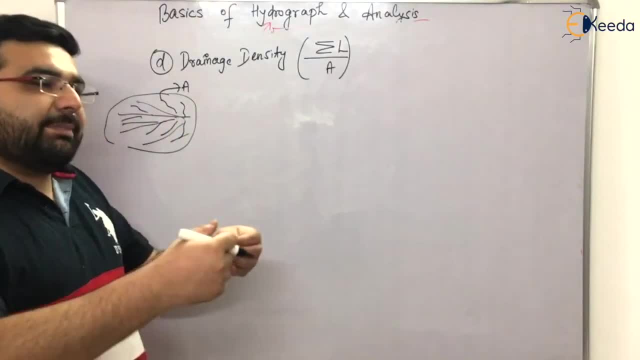 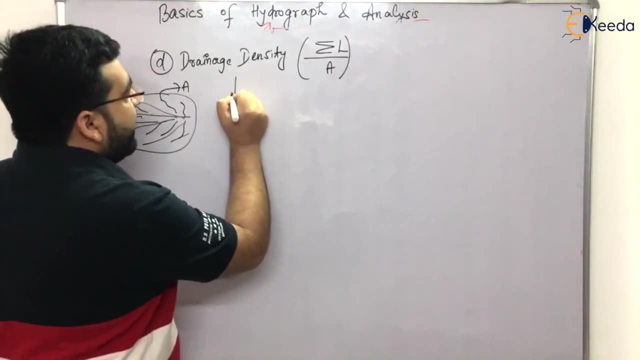 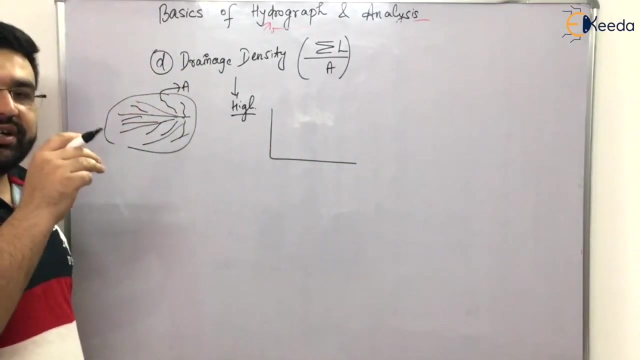 has happened. so the whole of the water will be dissipated quickly by the streams. it will be dissipated very quickly. so i will say that if the drainage density is high, if it is high, so the peak discharge. you can say: if the drain density is very high, so the peak discharge. 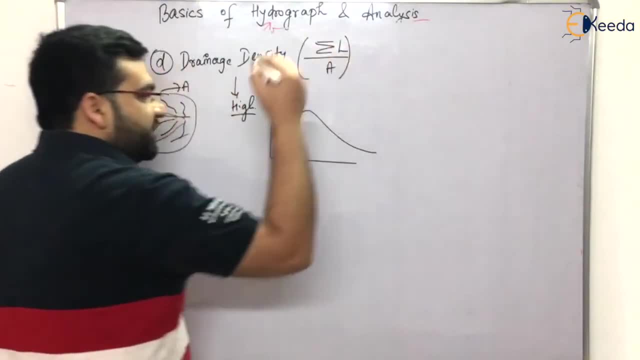 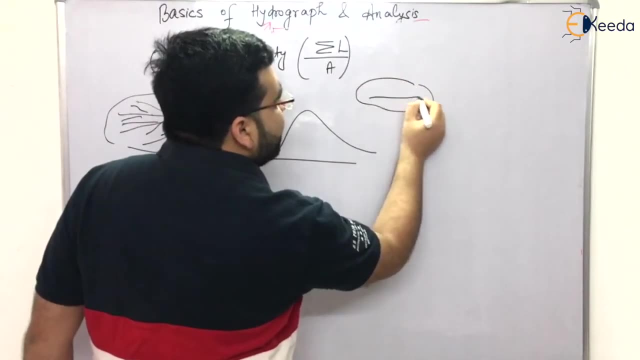 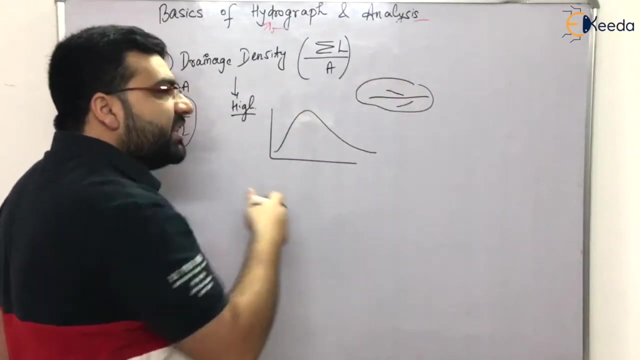 will be very high, like this clear. but if the drainage density is very low, let us say you have a catchment, only one stream, two stream and three stream. so what will happen? if a lot of you can say precipitation has happened over this particular catchment area, but there 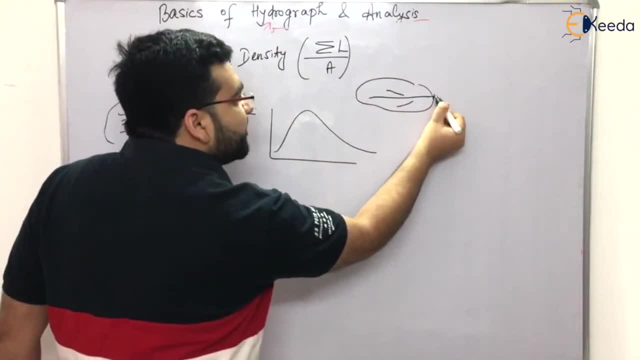 is no source to carry that precipitation to some place. if the drainage density is very high, then what will happen? if there is a gush of water and if there is a lot of precipitation, this goth station. there is no source. it will take a lot of time. so the your 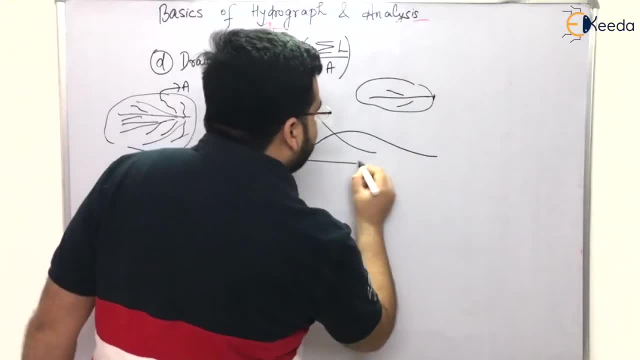 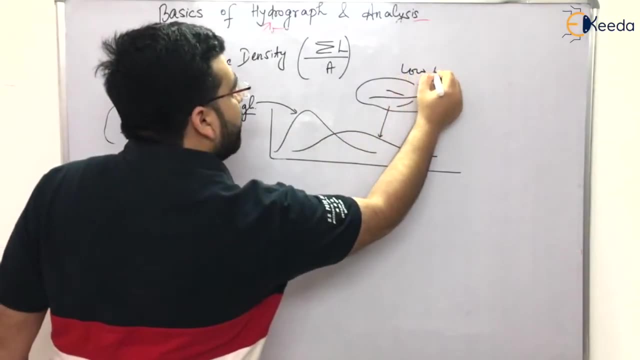 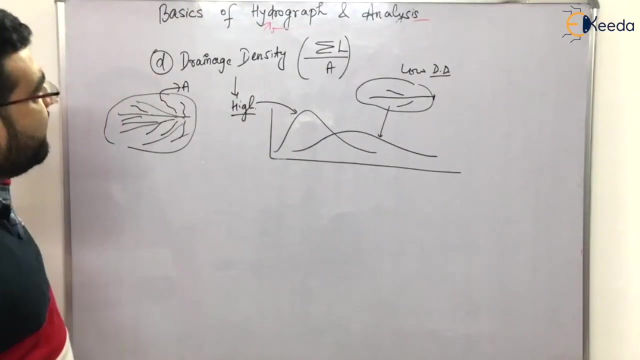 hydrograph would be like this, like this. so this is for this and this is for the high drainage density and this is for the low drainage density. low drainage density- DD means drainage density- yeah, so this is the fourth factor on which the hydrograph it actually depends. yeah, now the next factor, fifth factor in which 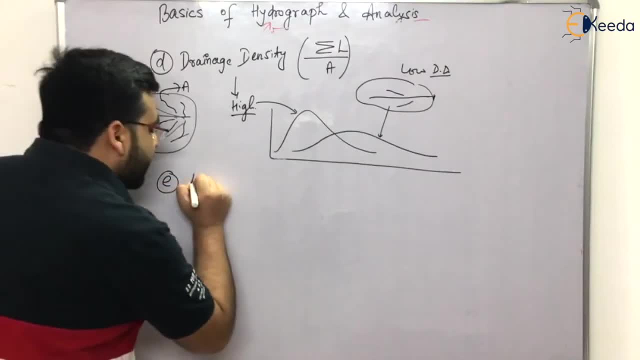 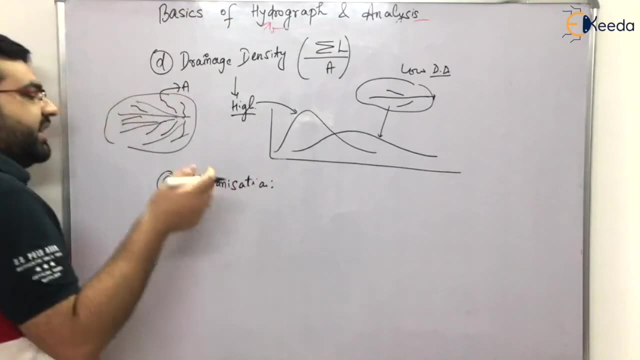 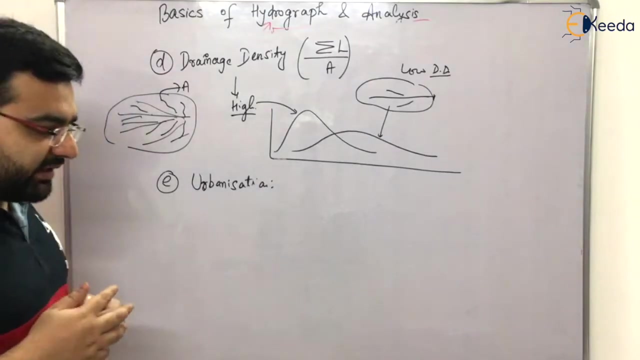 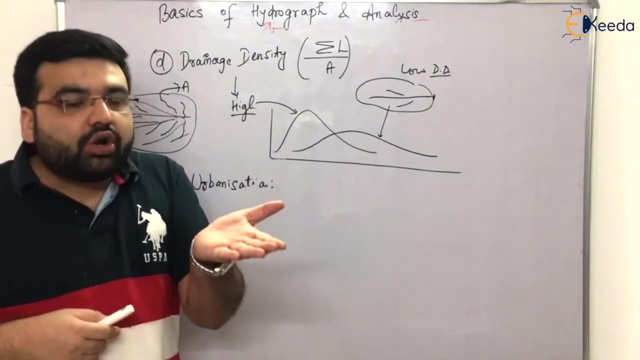 on which it depends, which has been asked in examination, is urbanization, urbanization. urbanization means earlier there was some village and now we have, you can say, developed that particular area into an urban area. now you tell me one thing: whether an urban area has, you can say, a virgin land more or a rural. 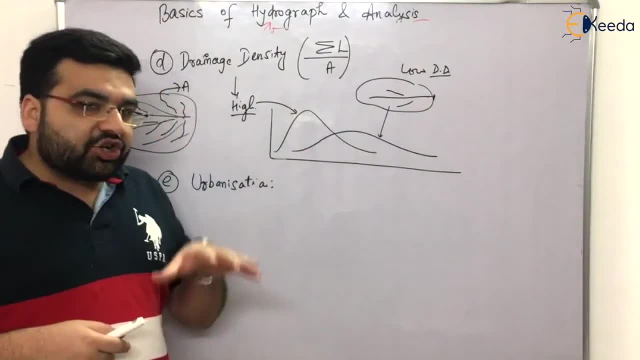 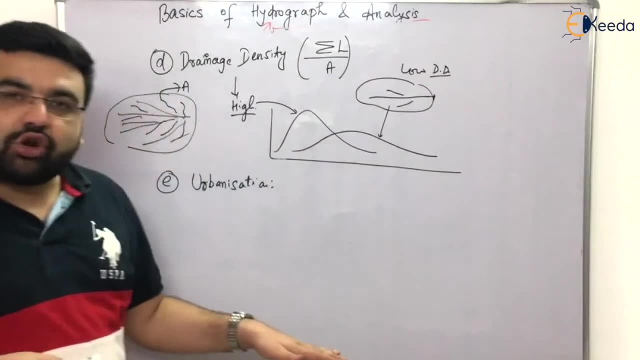 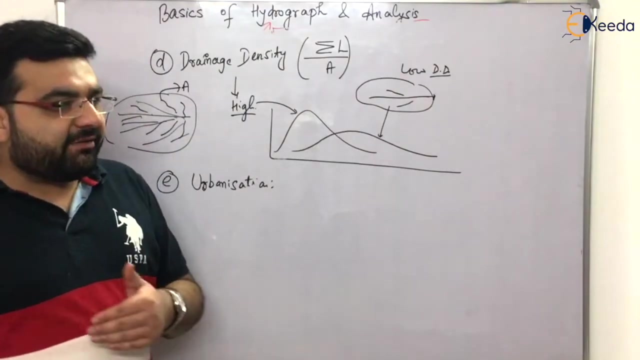 area. let me again repeat it now: in rural areas you can say an urban area has, you can say, a virgin land more or a rural area. you must be seeing that the you can say the proper finished concrete area is very less. in rural areas most of the area is proper ground. we have farms right, we have fields. 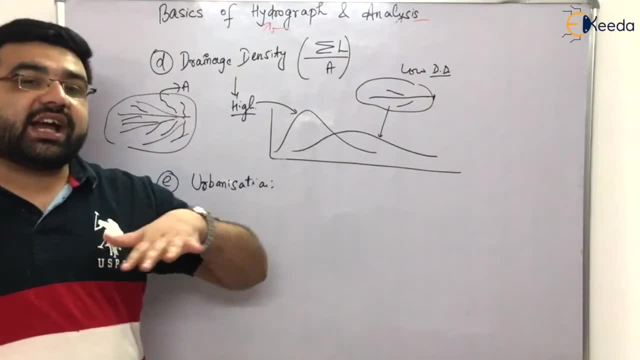 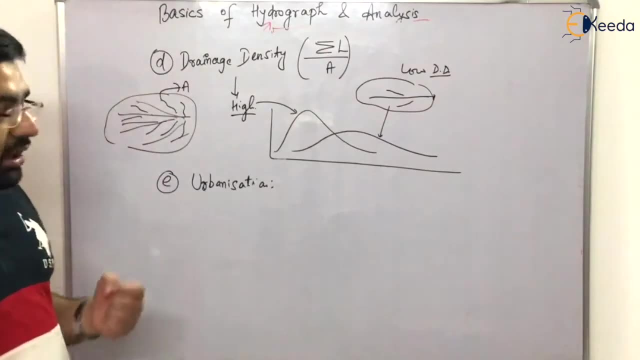 agricultural fields. right, so not much of the area is totally covered with concrete or it is not a very tough area, right? but as far as the urban urbanization is concerned, urban areas are concerned, we have roads. we have metallic roads- right now we have, you can say, 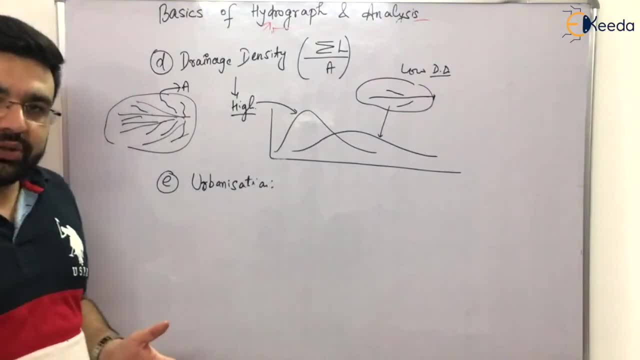 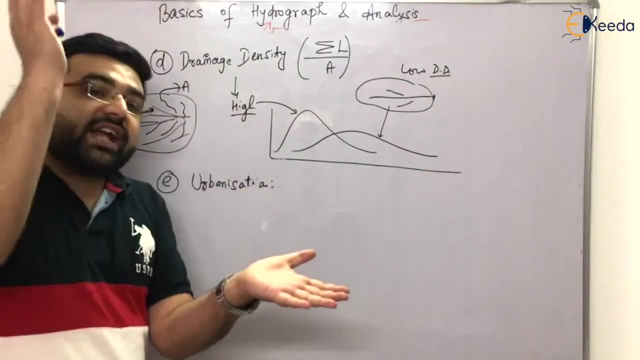 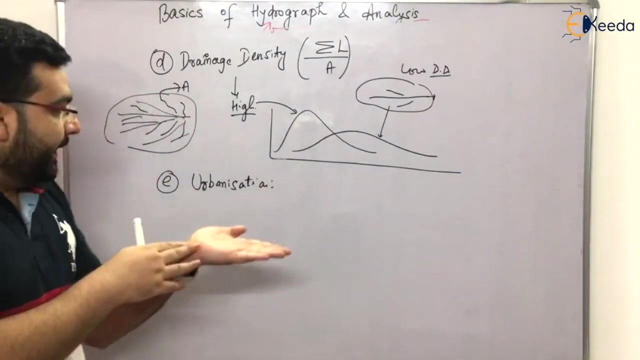 societies also. we have, you can say, finished floors also, right. so what will happen is that the upper surface of the ground, it will not be in directly contact with the- you can say particular storm or precipitation. so what is there? we have a. you can say there is a. 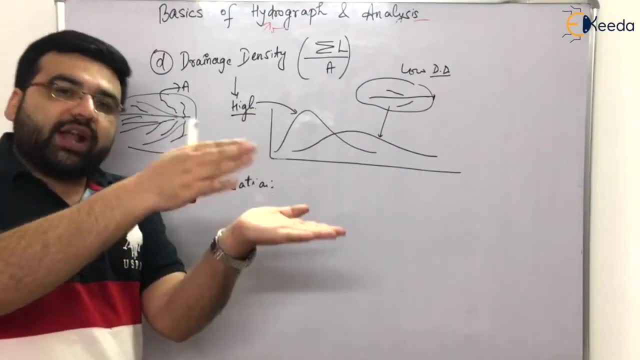 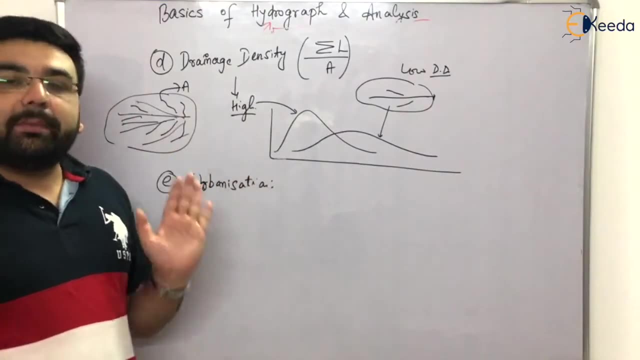 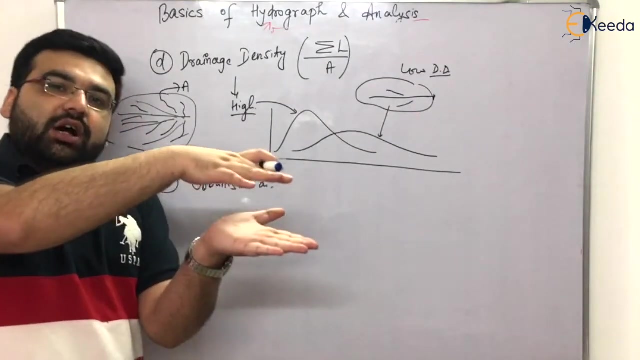 barrier of concrete or metallic road or anything. so I can say that if the urbanization is more so, the infiltration will be very less because the, the rainfall or the precipitation is not in directly contact with the earth. it already has some some something over it. it can be a metallic road, it can be a house or it can be anything. 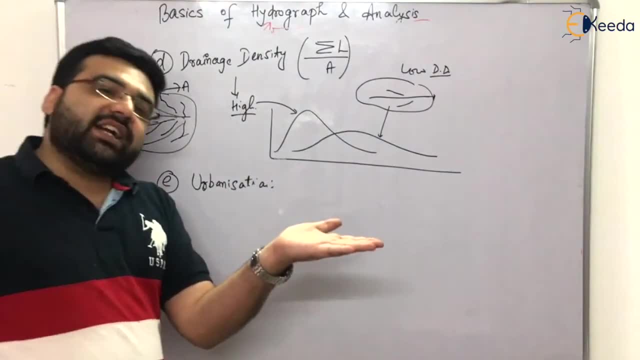 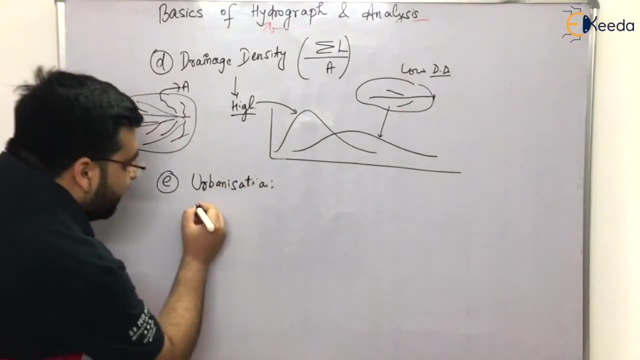 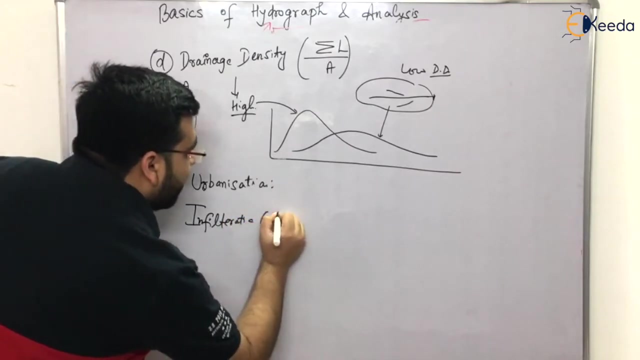 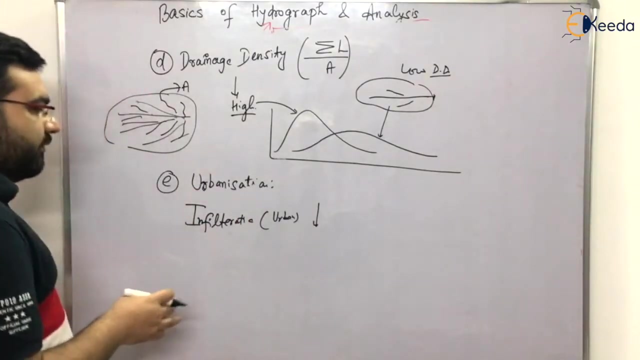 right. but in case of a village area, the surface, it is directly in contact with precipitation, the it meets with precipitation directly. so I can say that the infiltration, the infiltration in case of an urban area, is very less because there is no ground, there is no land which is available for infiltration. 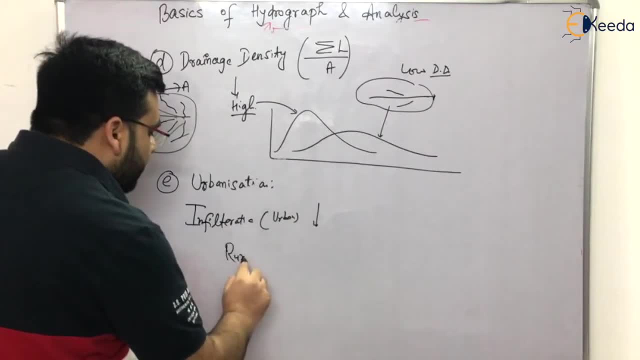 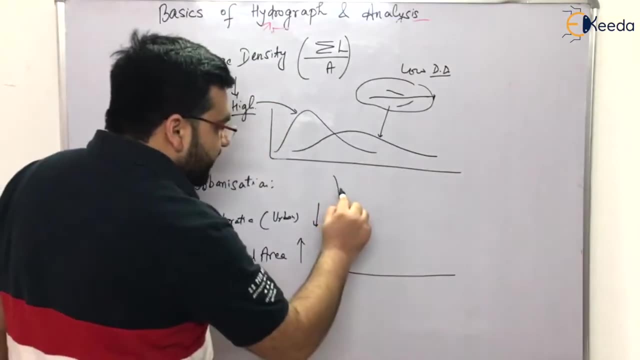 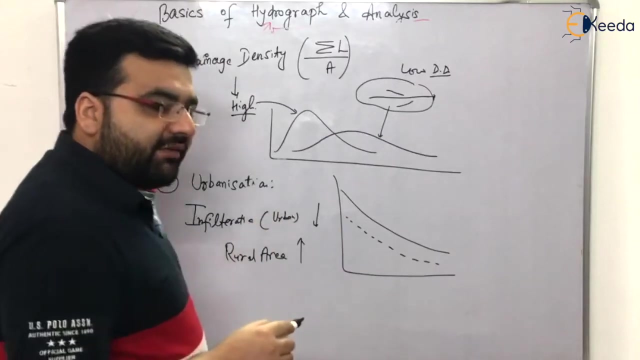 and for rural area. rural area it is high. so if I draw a graph, it will be like this. so this is before urbanization and this is after urbanization, right before urbanization and after urbanization. this is your infiltration, infiltration, this is your time t. so this is. 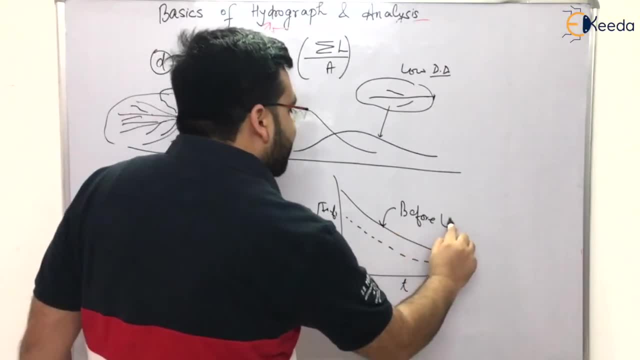 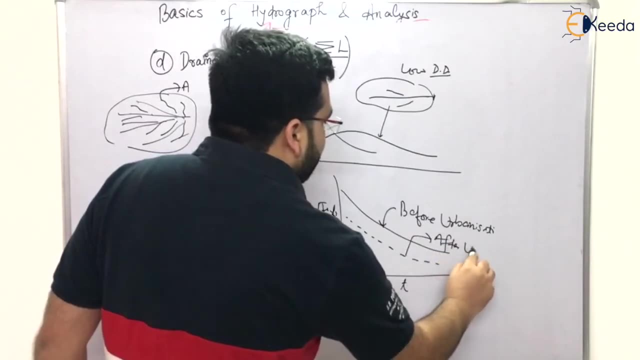 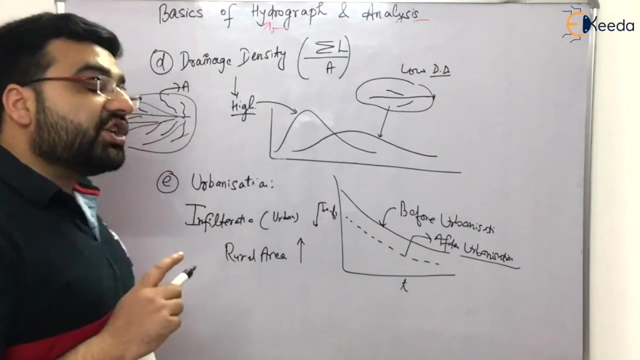 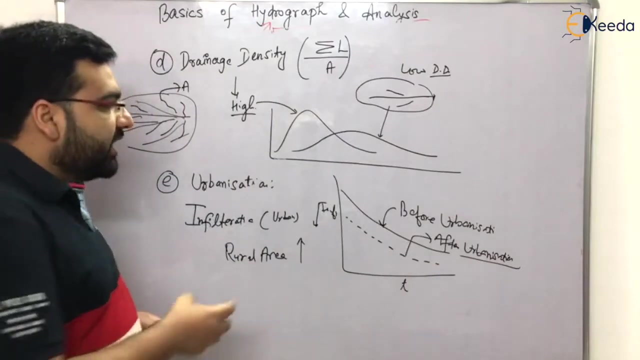 your before urbanization, urbanization. and this is your after urbanization, after urbanization. now, if the infiltration is less, if the infiltration is less, what will happen to the discharge? will it be more or will it be less? it will be more right, because only a few water, only few water can. 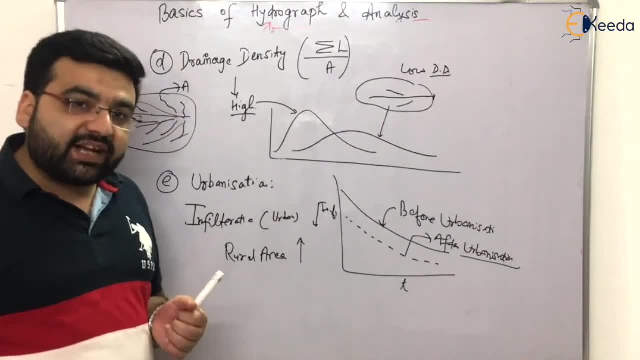 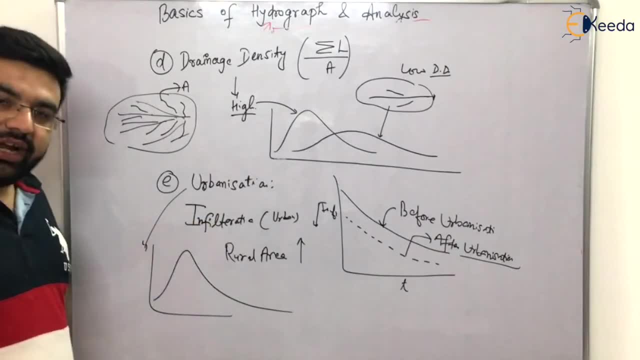 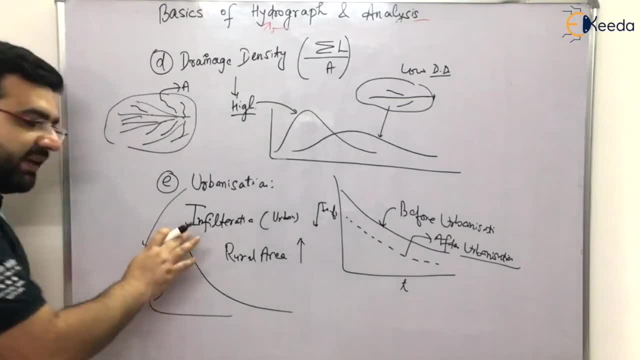 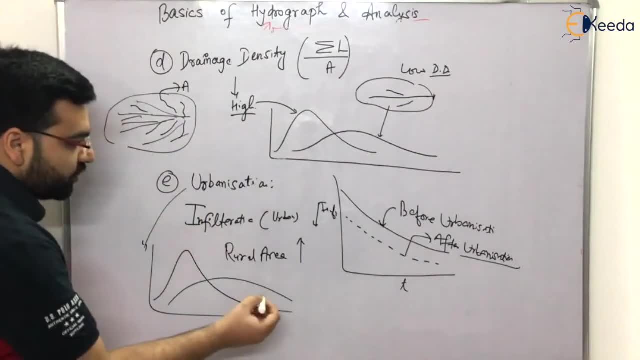 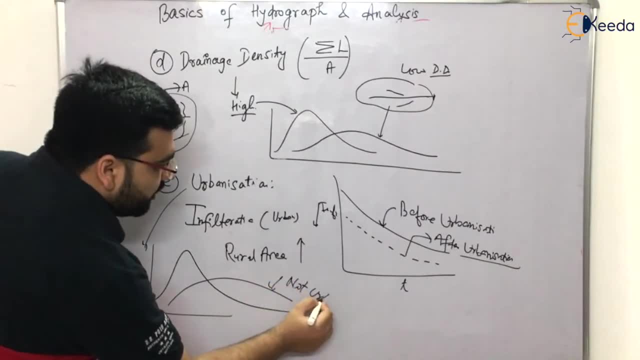 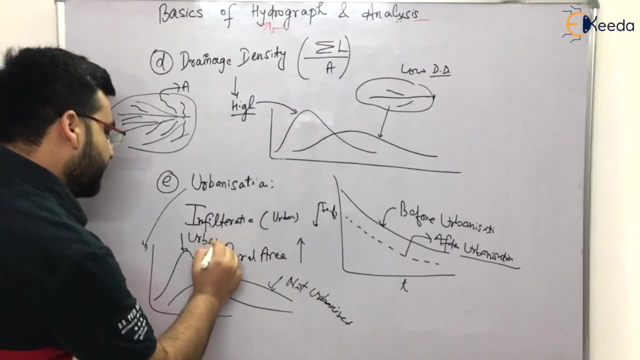 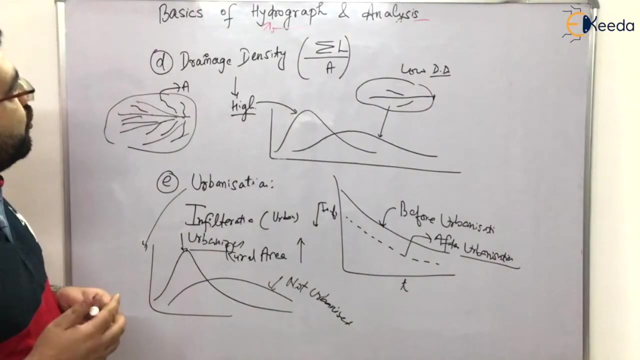 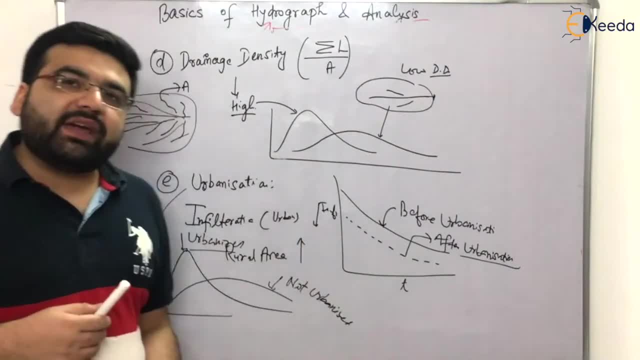 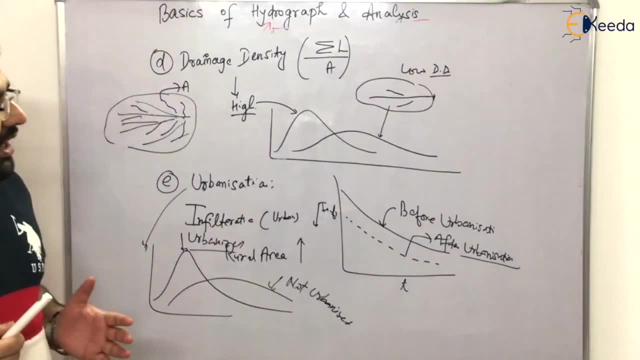 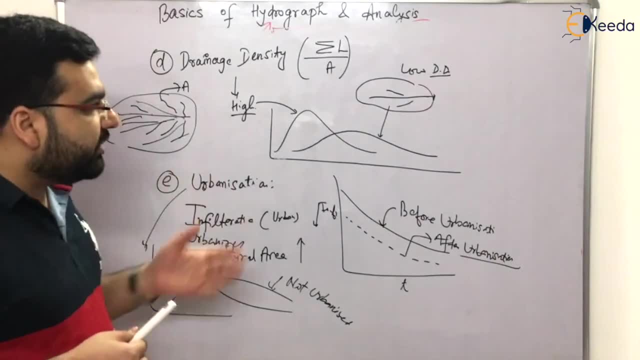 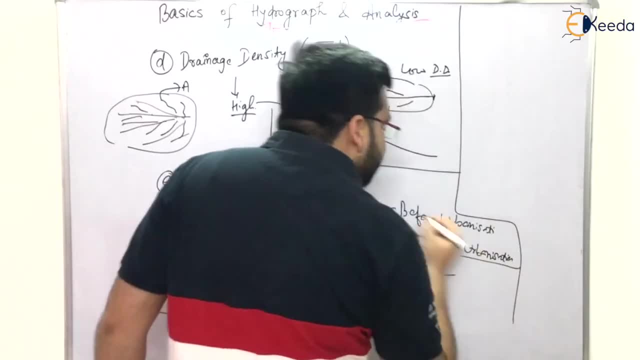 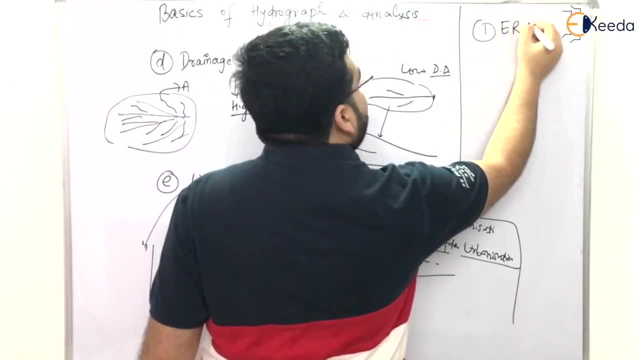 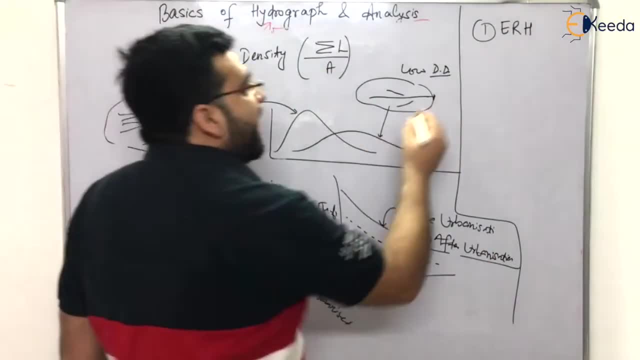 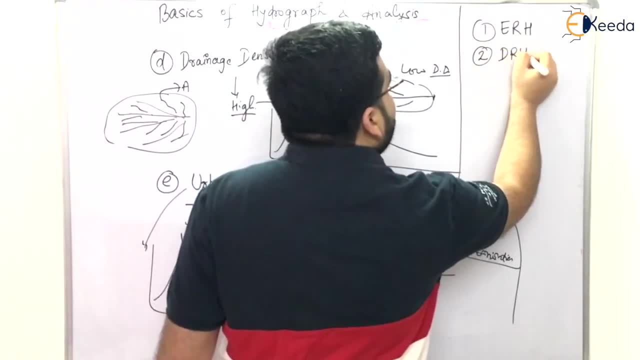 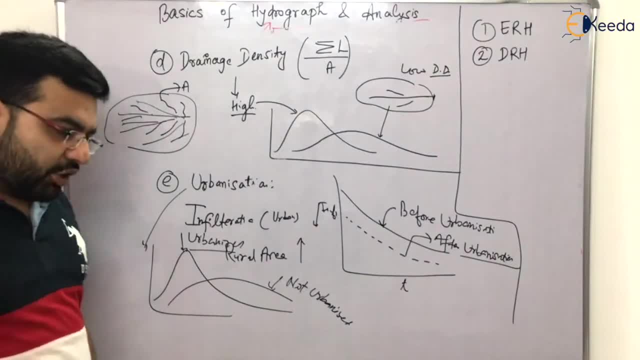 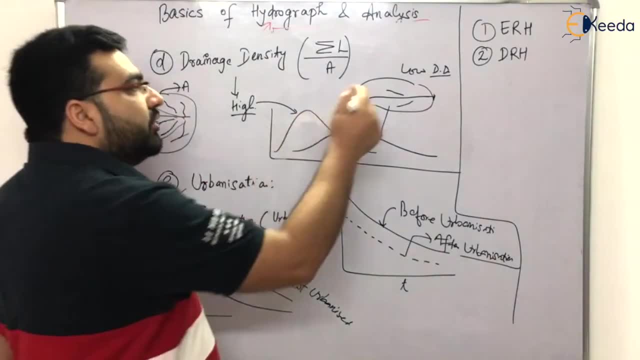 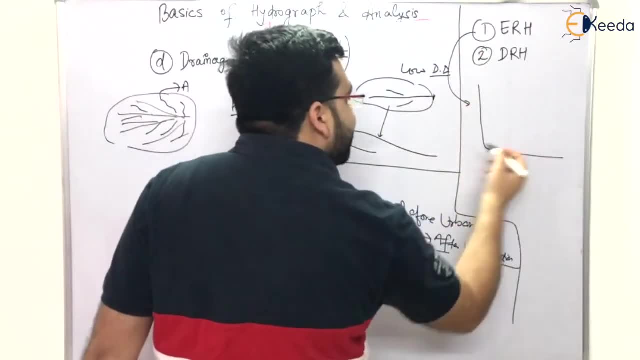 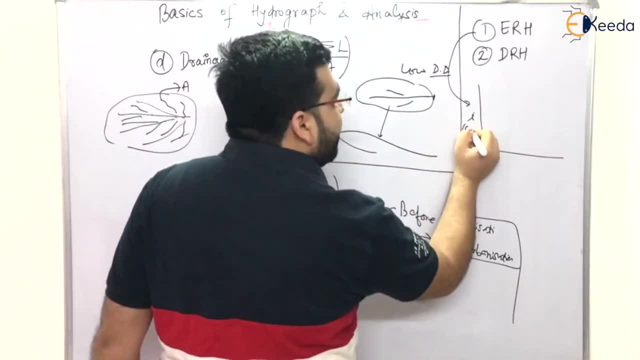 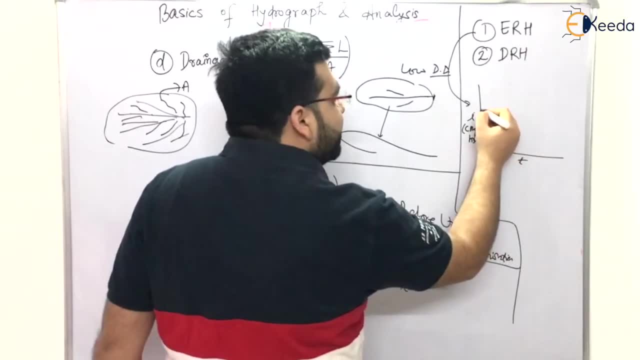 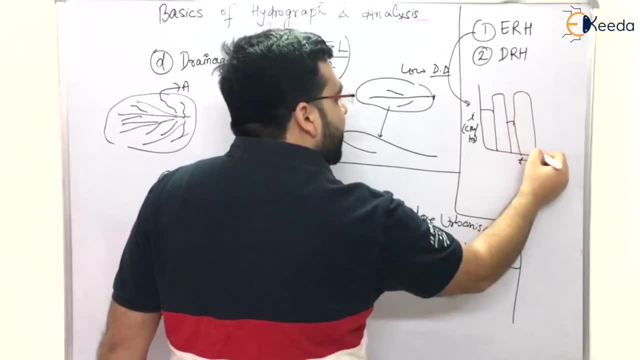 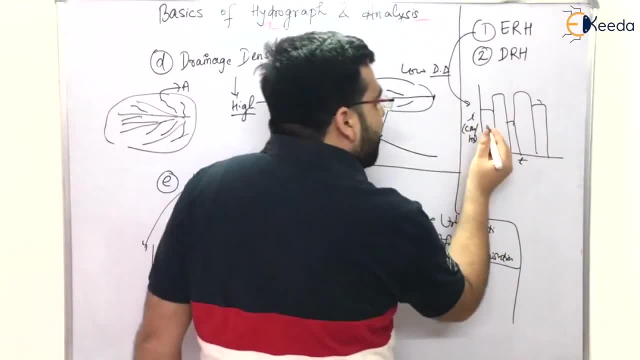 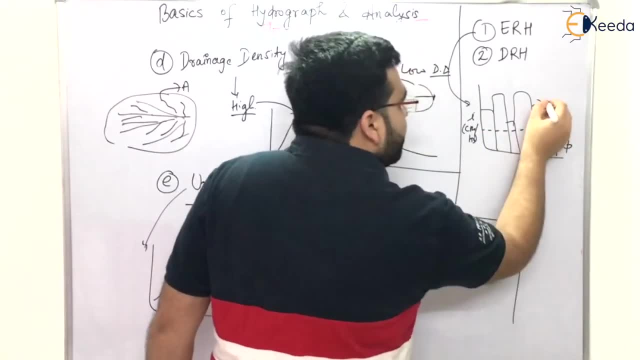 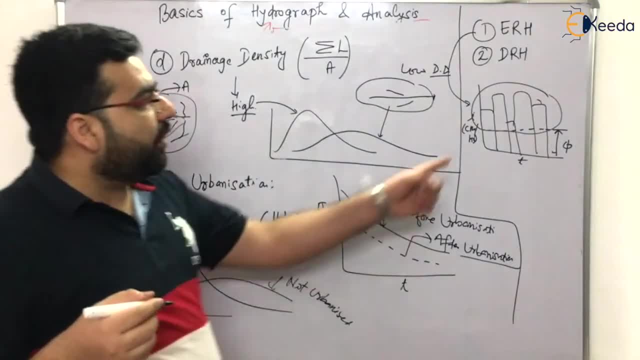 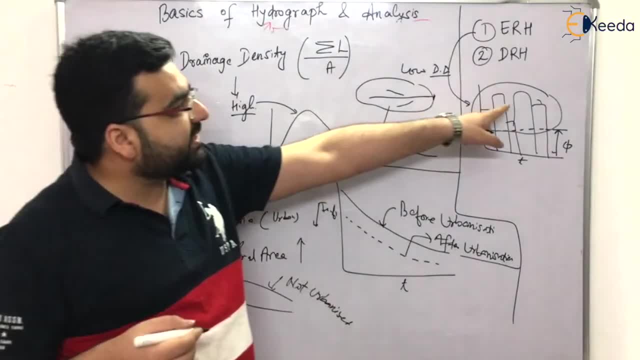 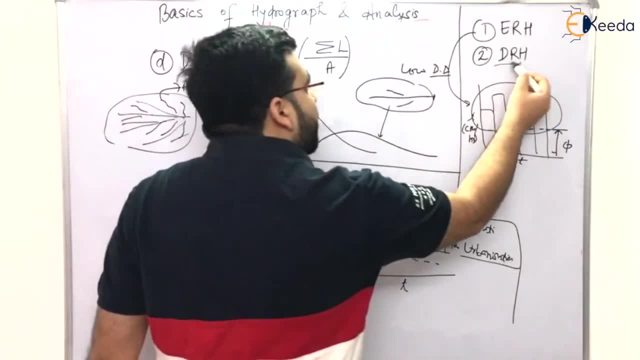 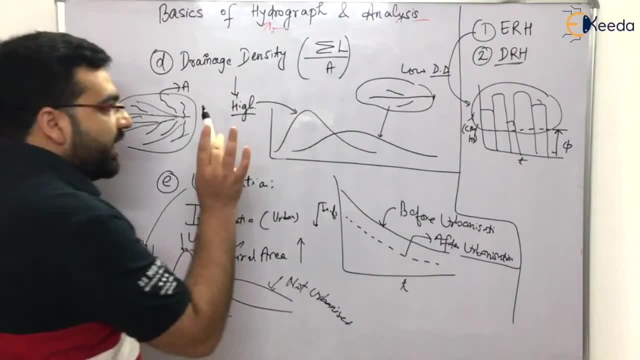 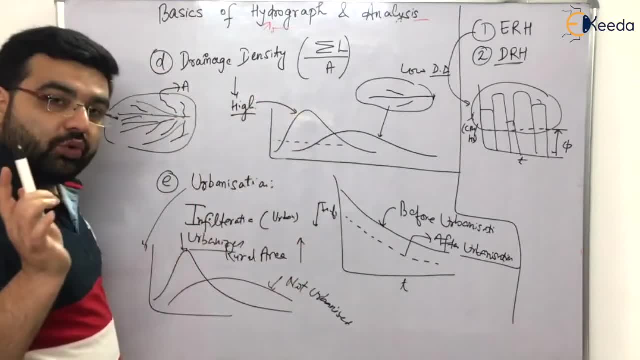 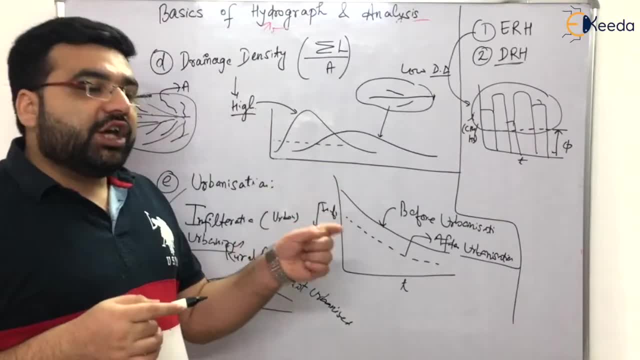 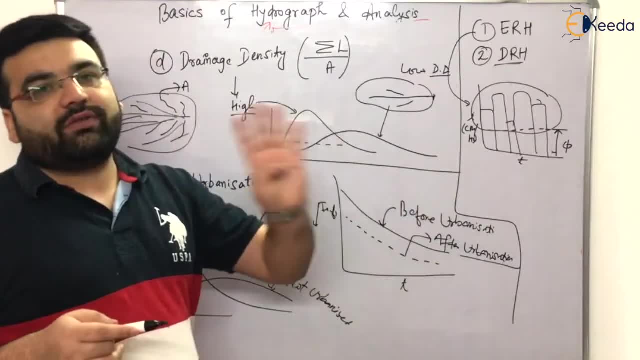 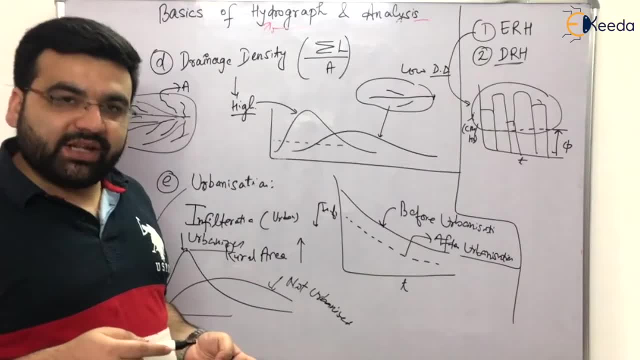 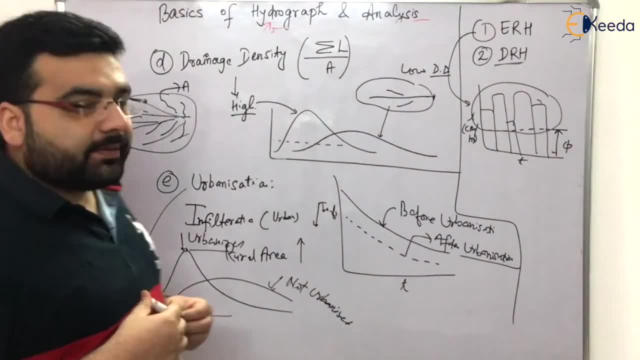 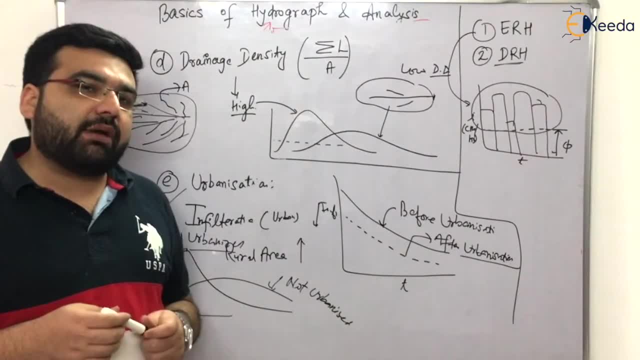 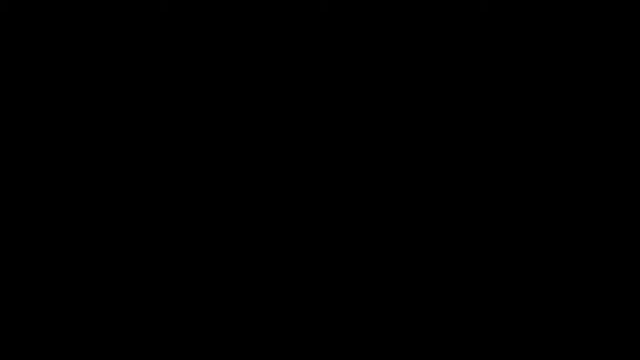